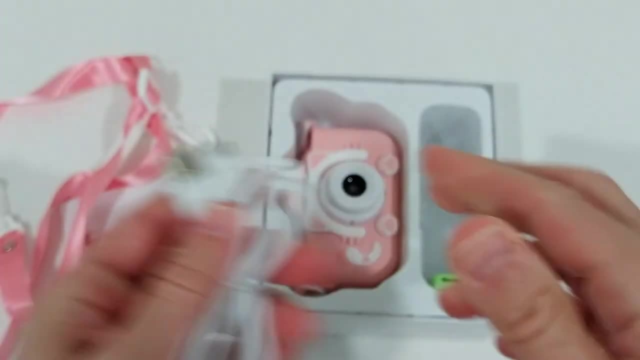 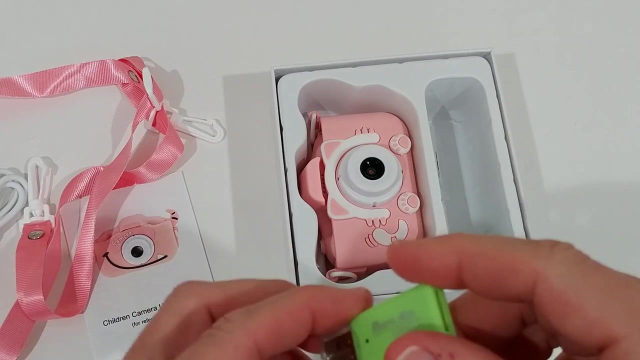 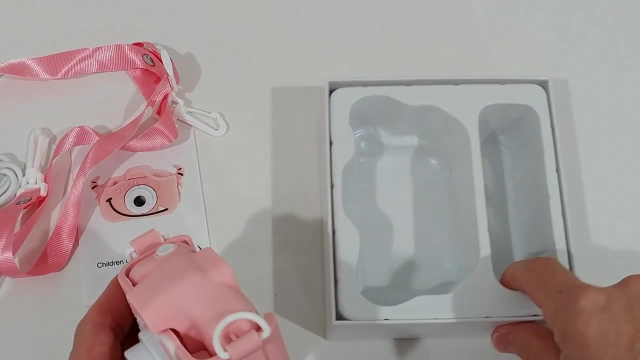 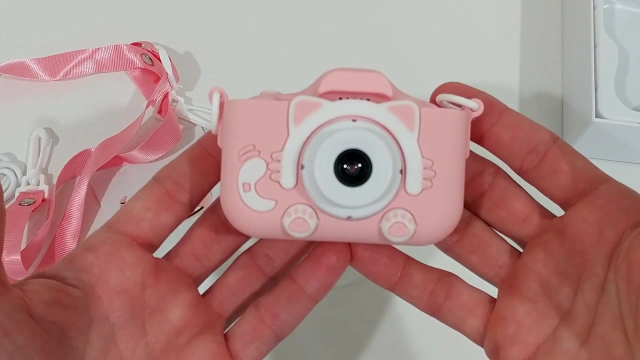 It's micro USB charging cable. We also have the USB stick. Yeah, that's an adapter for the micro SD card or SD card, whatever it is. Here we have the camera. It's pretty small. I mean small. I would say it's about the right size for small children, Not too big, not too small. Here is how it looks. Also comes with a. 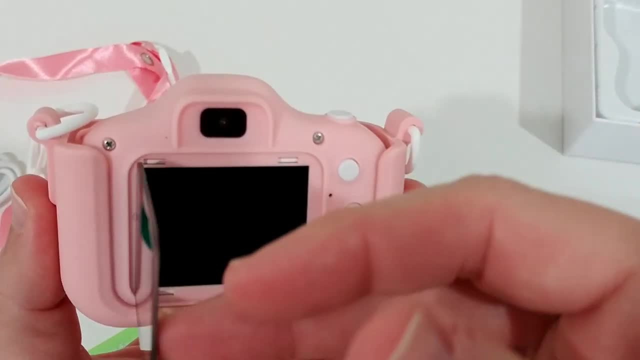 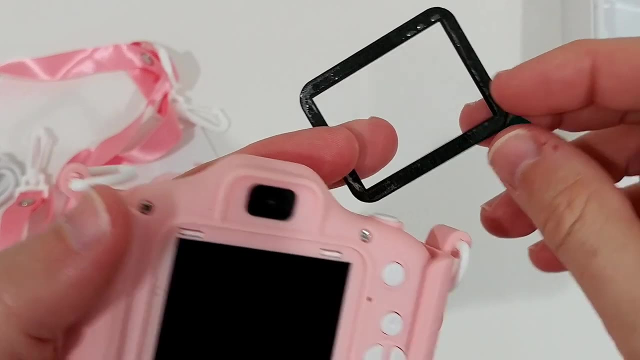 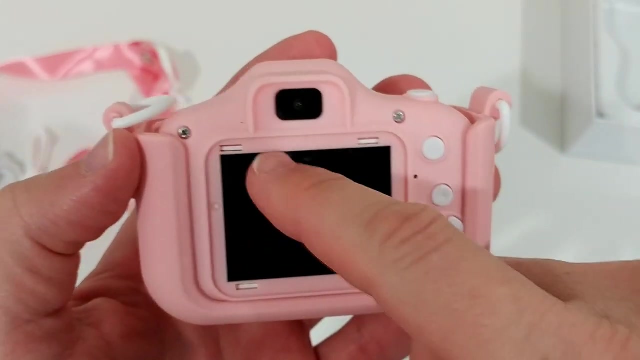 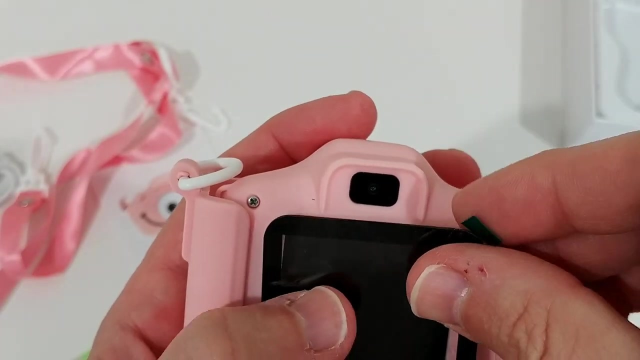 protection on the back. What's that? Yeah, I'll have to figure out what that is. So it looks like the glue comes already off. It's some kind of protection, probably because of this screen. Yeah, the screen itself is probably really thin, So they added this protection here, which is a nice idea, but it definitely should. 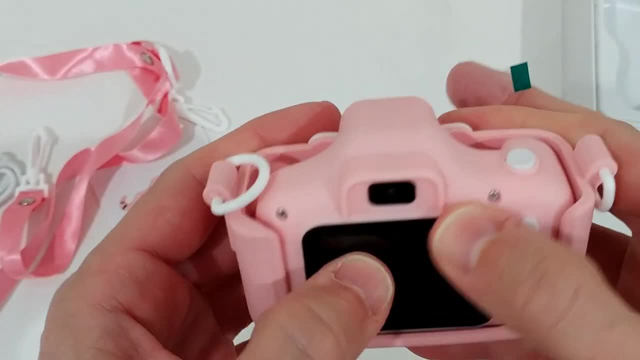 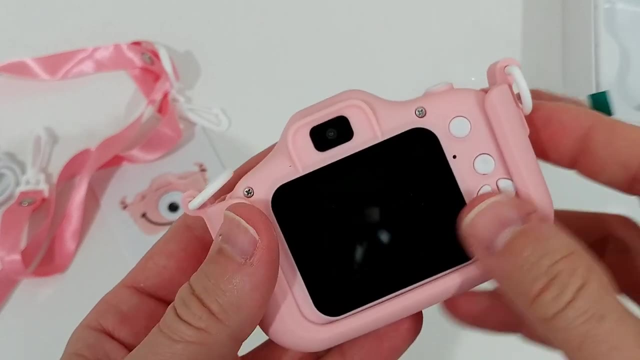 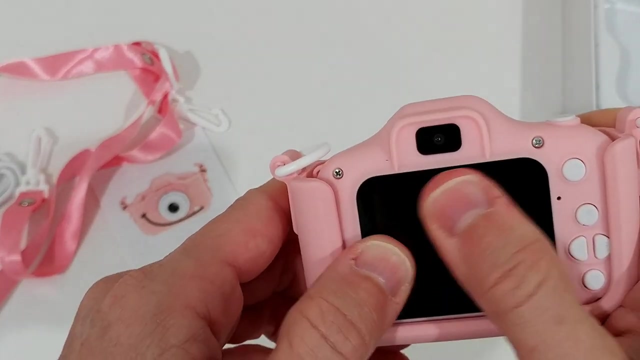 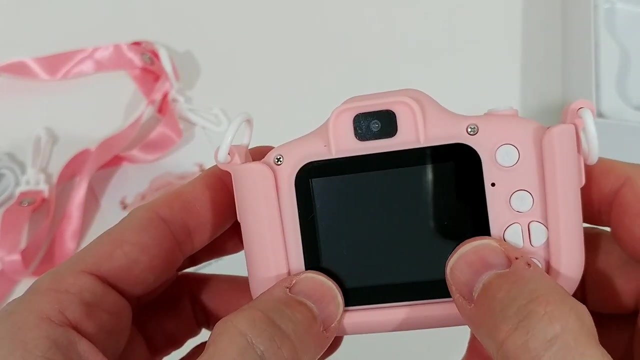 stick on that. I mean you can press it back and yeah, it looks like it's holding up, but it was not so nicely done. I mean you can see? yeah, you have seen the glue. I mean you can always put it back, but yeah, it should stick from the beginning. That's a little bit disappointing But, apart from that, looking good at the moment, It's about what I was expecting. 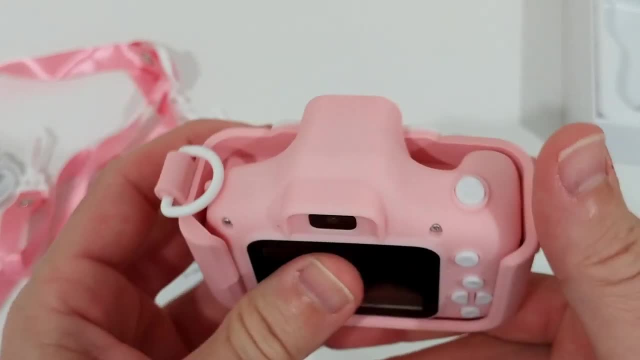 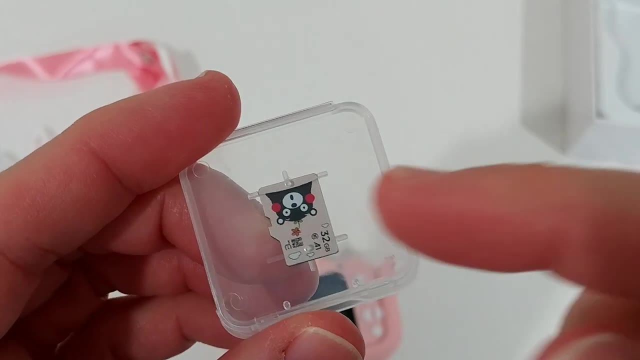 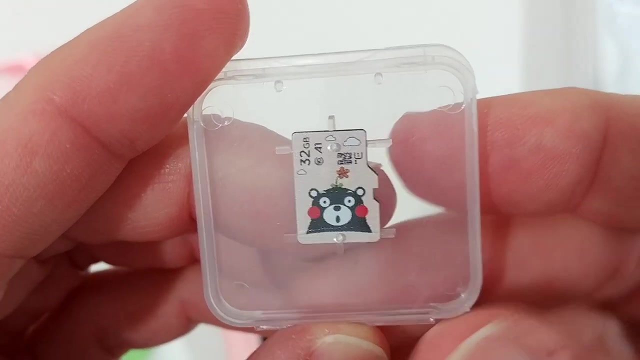 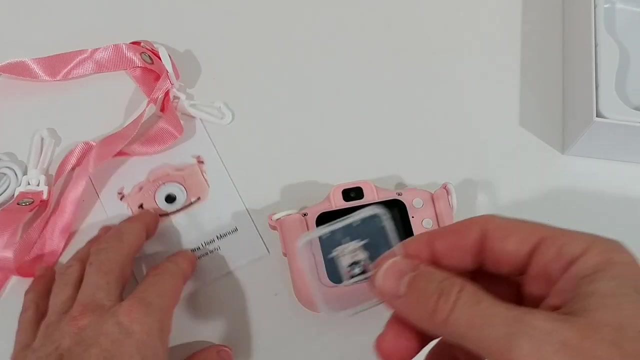 I don't know if we can take this out. So yeah, I'll check a little bit with that and I will charge it and insert the micro SD card. Yeah, look at this thing, Isn't that nice thing. It's the most beautiful micro SD card I've ever seen. And 32 gigabytes, That's quite a lot. I mean, you can already pay a lot of money for something like that and you get everything with the adapter. 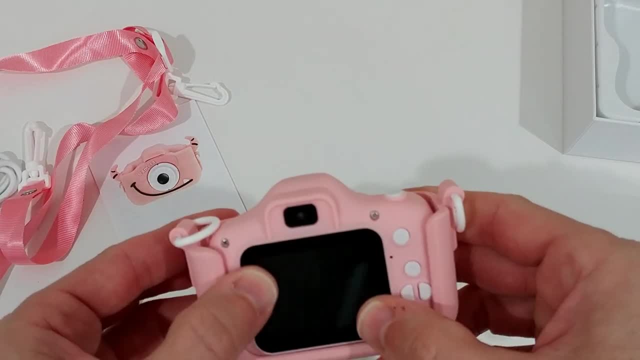 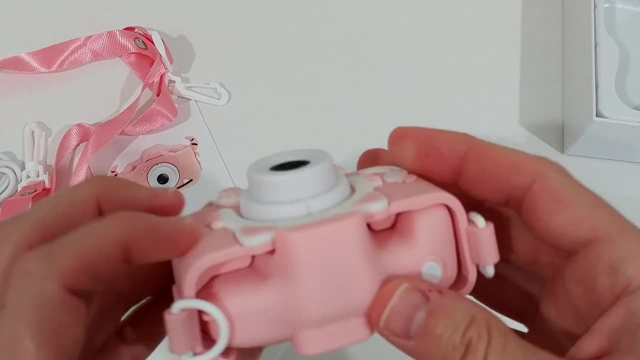 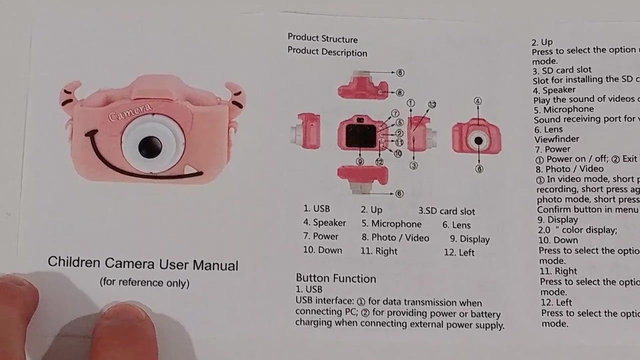 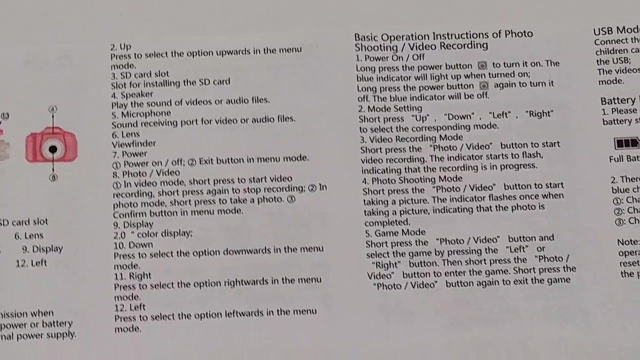 And yeah, as long as we keep this protection keeps sticking, I'm not worried about that. So, yeah, I'll charge it and test it and let you know. So of course, I'll do what I always do, And that means I'm going to show you the instructions really quickly So you get the opportunity to read everything clearly. 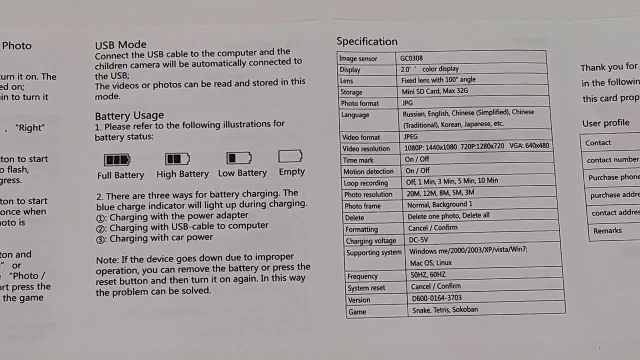 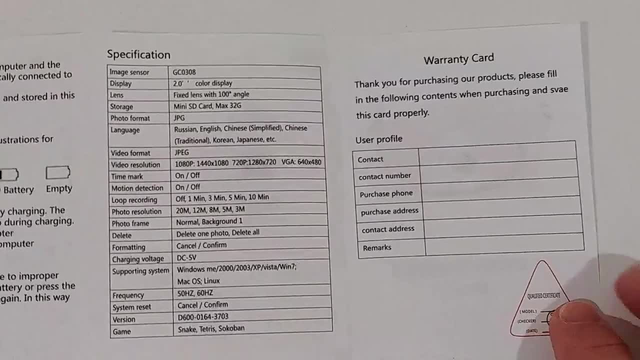 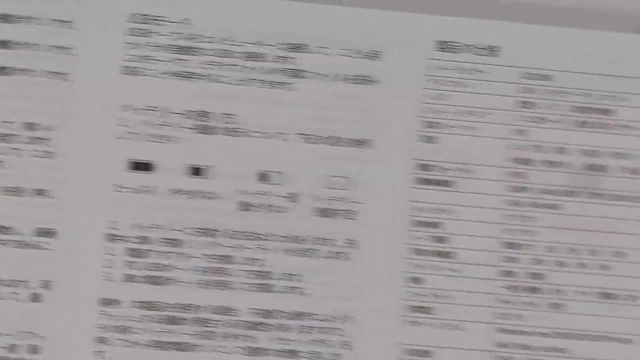 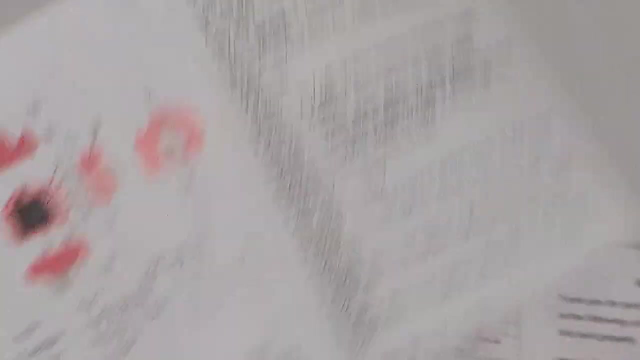 That's not everything on Amazon and you probably won't find everything online. Usually these cheap manufacturers, they don't have even a website or it's hard to find it. Here's already everything, the full instructions, because the backside is everything only Chinese. So you can see, it's pretty, pretty simple And I've already been trying a little bit around. not the full thing, but it definitely. 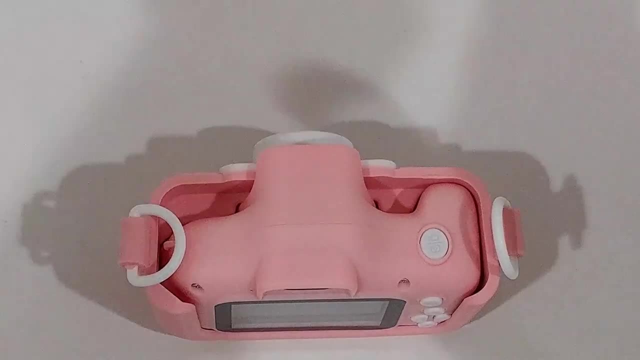 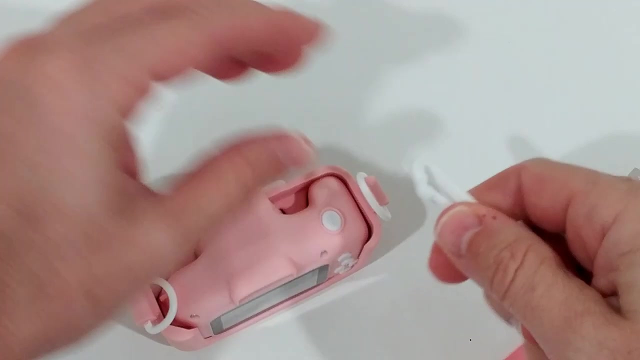 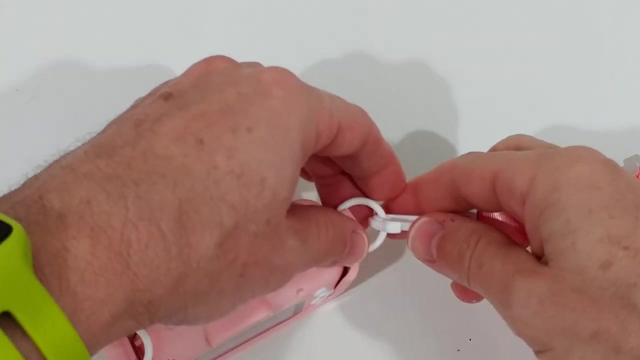 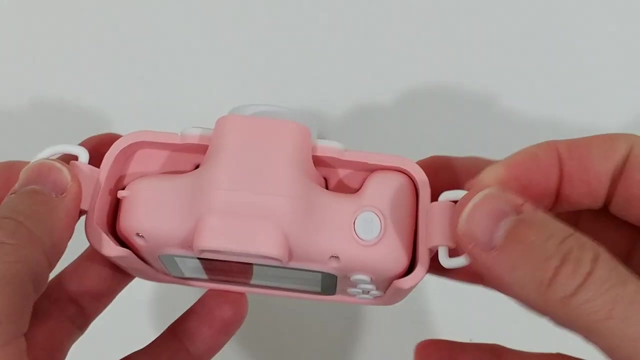 looks pretty easy. So actually at the moment I'm pretty excited about that, But let's see then in detail. Of course I will show you the footage and everything you can see. You can hook this strap up so you can secure it really nicely. The good thing is it's secured in this like case, some kind of case, and the case makes sure it's protected. 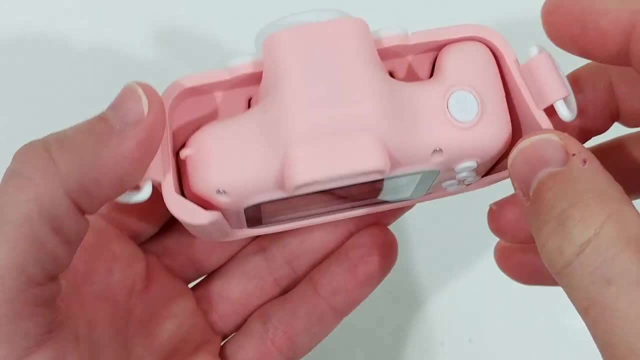 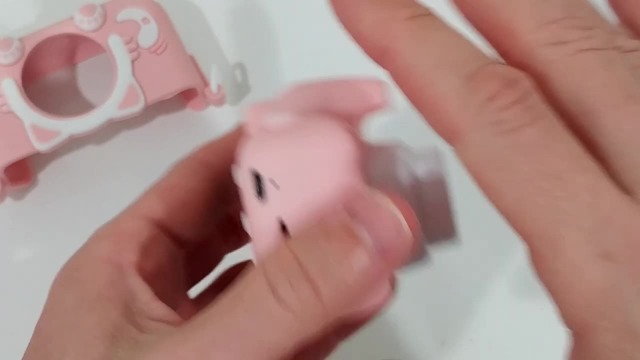 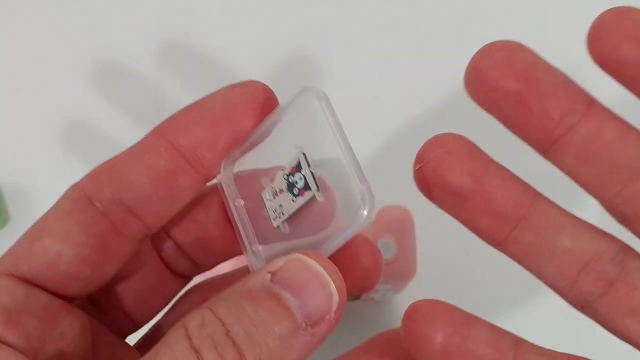 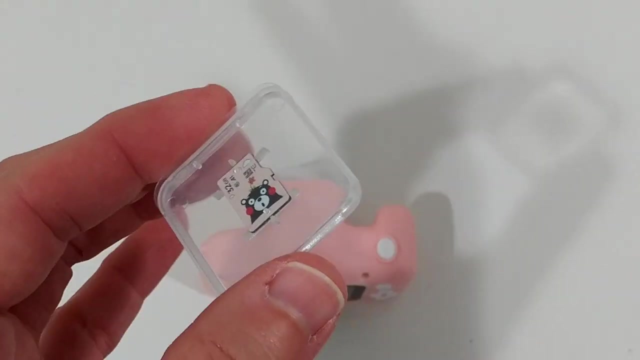 A little bit regarding charging and micro SD card slot, But you can easily take it out if you need to do something with the micro SD card or charge, So you can easily hold it like this. First, of course, we have to insert the micro SD card. Without the SD card, absolutely nothing will work, So let's do that now. Okay, I've already done it for the first time To show you the 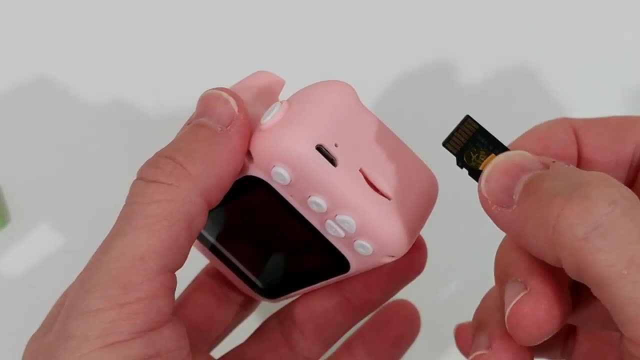 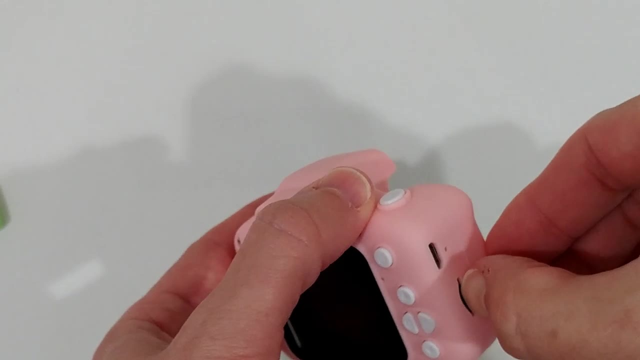 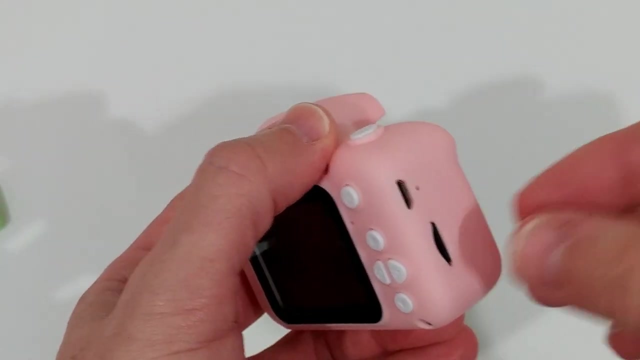 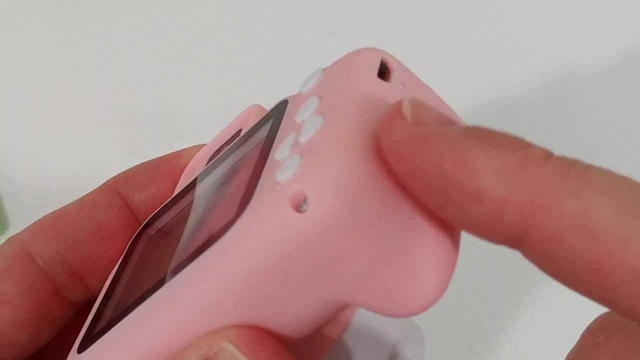 show you that I'll make it one more time. The pins have to go to the back, towards the screen, So you can use your fingernails or like a coin or something like that, And if you want to release it, give it just another push like normal. It's pretty easy and it's not elevated or something. It's absolutely flat, which is nice, But of course you can't be close. The only thing. 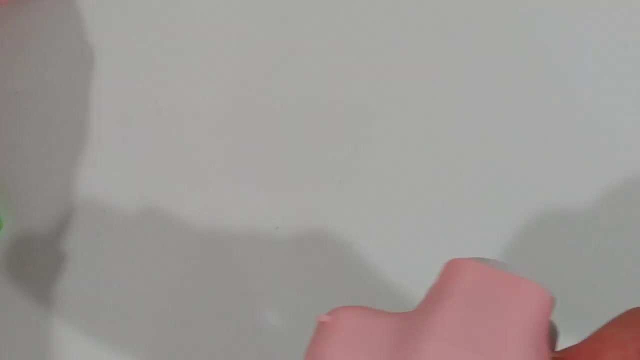 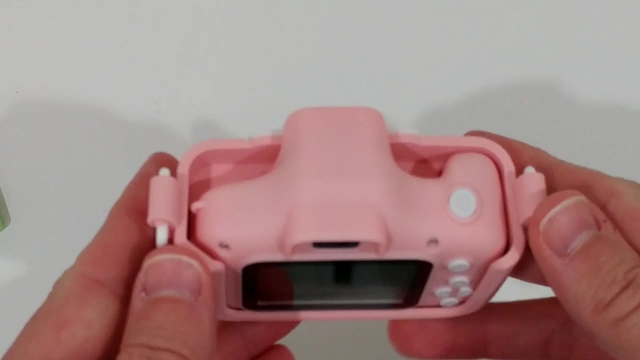 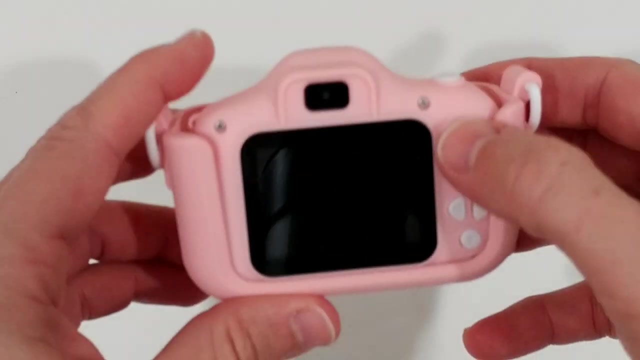 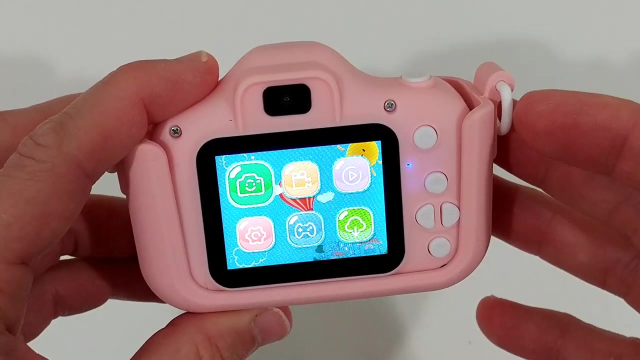 to protect. is this semi case or whatsoever? Yeah, let's put it back and pretend we're using it like a child. So to turn it on is pretty easy Here. we have to long press here And you can see already the screen. The screen is easy to read. It's very bright. I have no doubt that we can also. 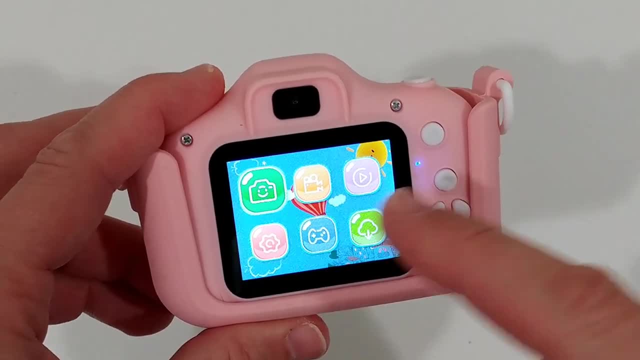 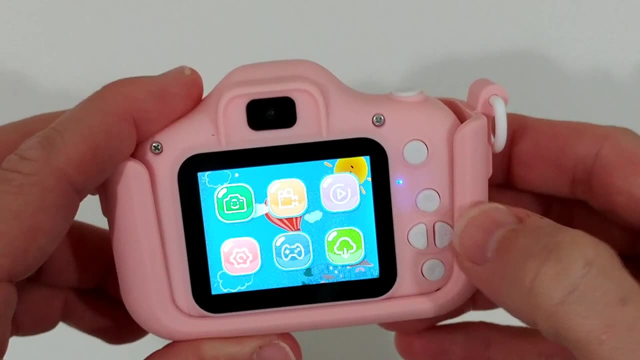 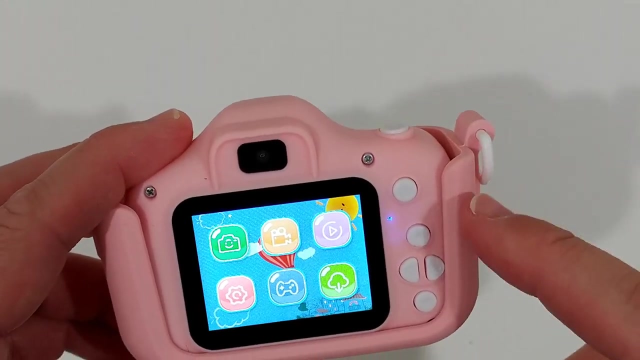 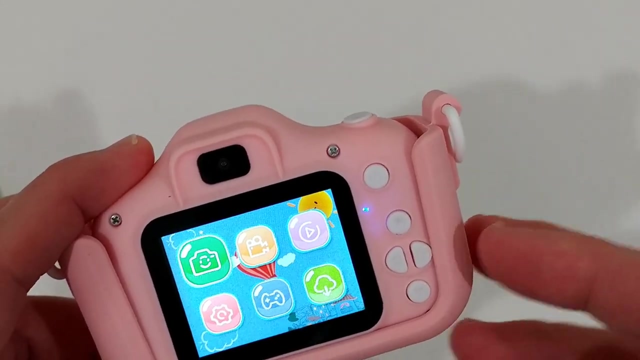 read it nicely or see it nicely outside. So there's no touchscreen, but you have these buttons here where you can move around easily up and down and left and right. So here's the camera and everything we want to confirm. we have to confirm here And this is the like, the back button. It's not described, but I found out this is actually like the back button. This is to confirm and this is also. 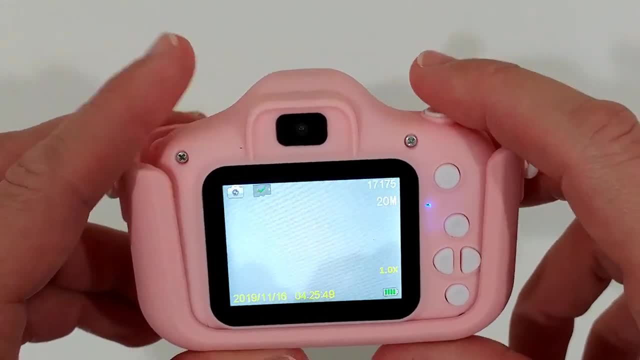 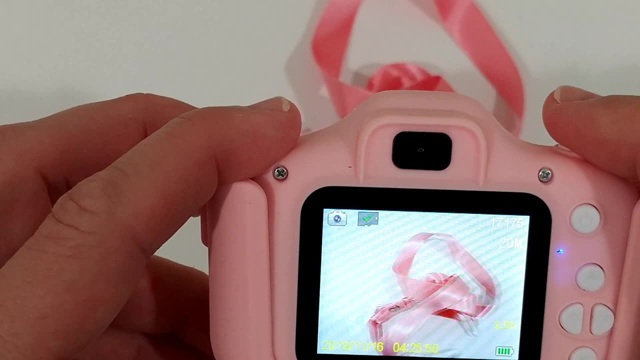 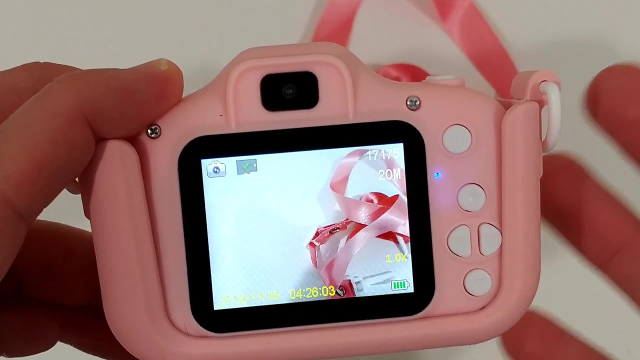 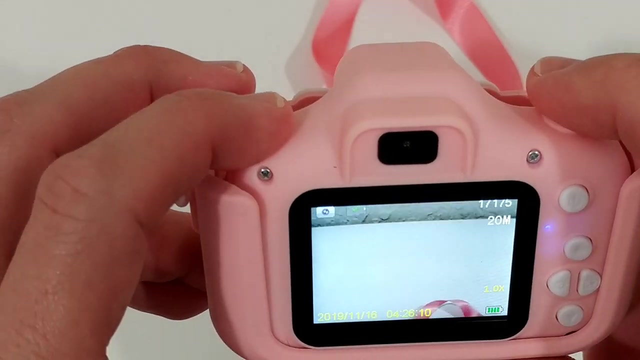 always back so we can select the camera and we can already output something here. So you can see that. And yeah, there is also like a little bit what you see. I mean, it's better than what you see. Of course, it's always difficult to record a screen with a camera. It's not perfect. The colors are good, It is. Yeah, it is not perfect. There are some lines going down. I've 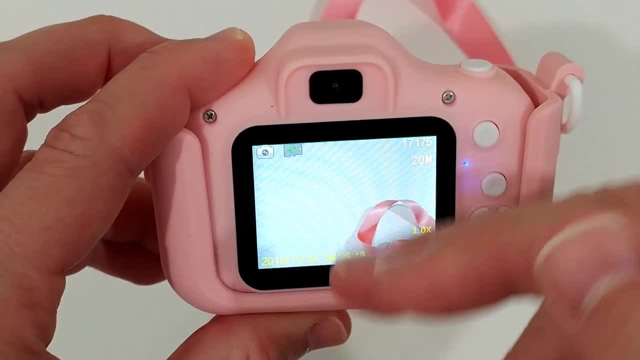 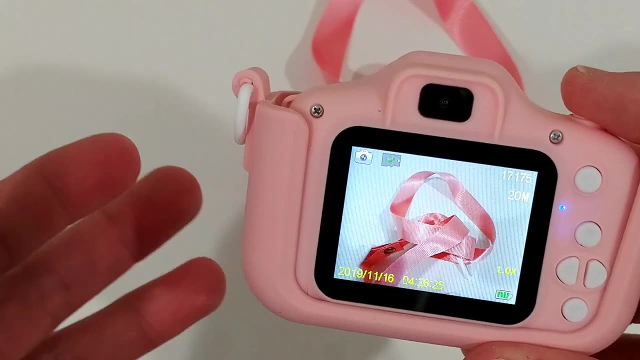 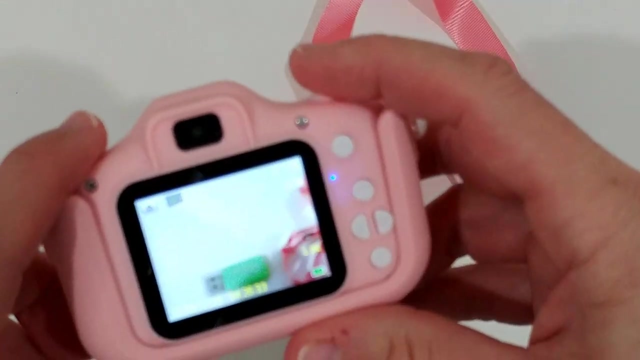 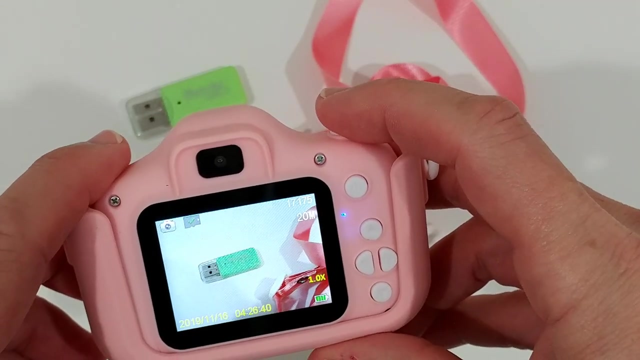 I think you can see that also in the camera: Some lines which are going down like small waves. Of course it's not the most expensive chip, not the most expensive screen, But you can really nicely see it like here. There's absolutely no problem with that And I think there's no focusing on nothing. That's just the Yeah, you can select the screen. 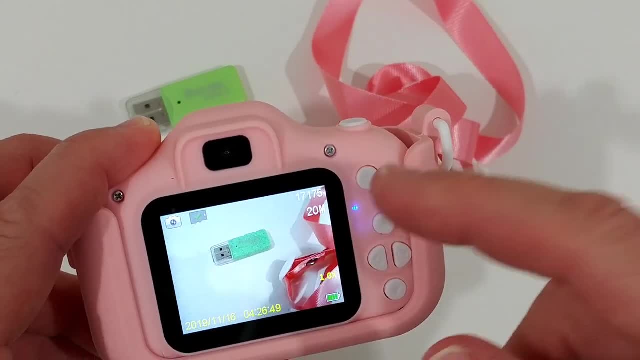 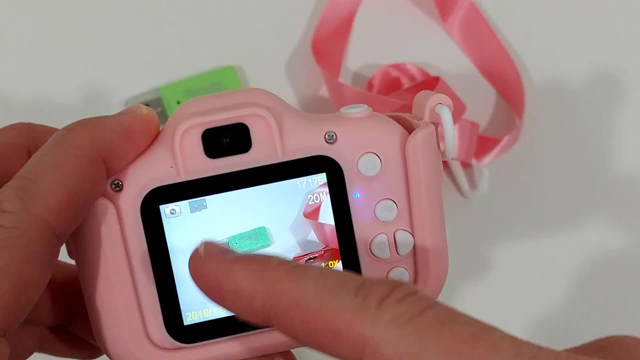 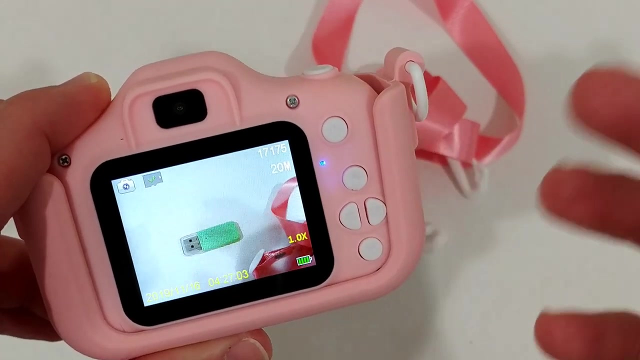 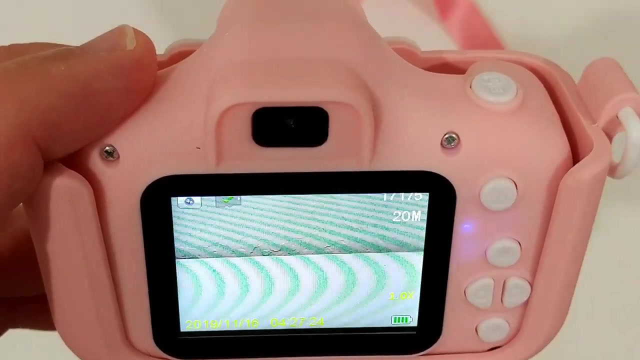 in the settings- I will show you that later on- that you can select that. you can see how many pictures there are left And you can see that's the picture mode. And we have the storage card inside. date and time will be printed on the picture. And here we have the battery, So actually everything, and there's even a camera to the back. I didn't know. I have no clue where it is, Probably it's here. I mean, that's not a viewfinder, It looks like. 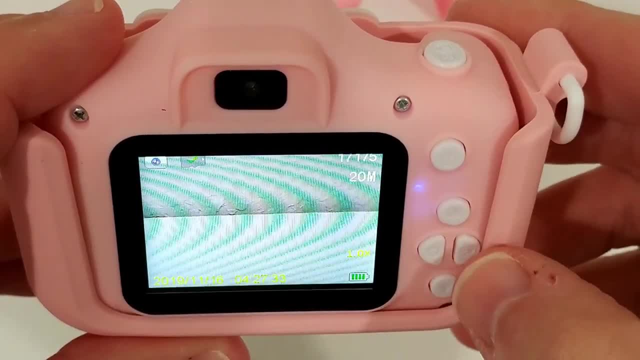 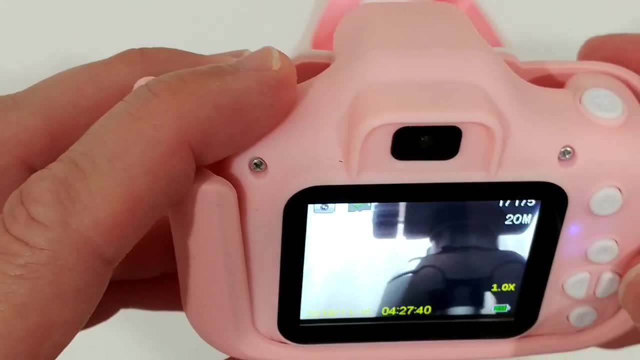 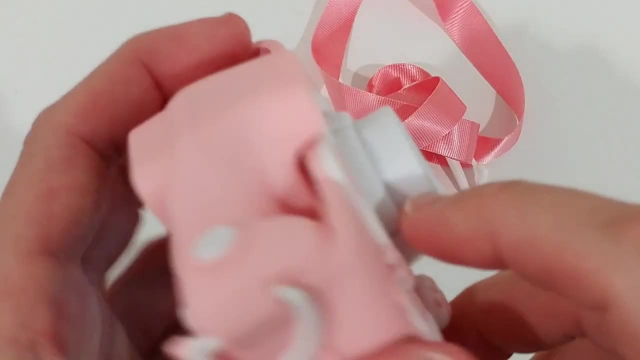 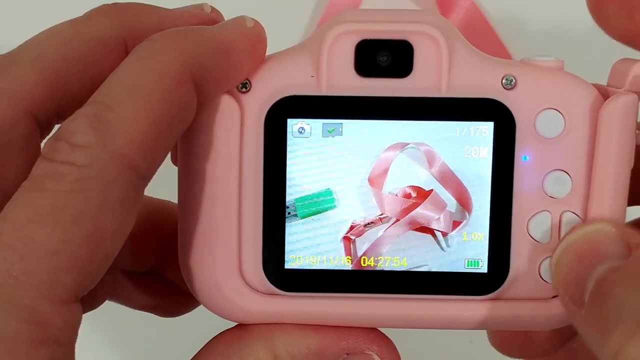 a viewfinder, but it's not a viewfinder. It's really interesting. You can switch the camera here to the back And, as you can see, that's me here with the tripod. That's pretty interesting here. So switch to the camera in the front, which is here So you can see. no, you find it, But that's actually a selfie camera here. That's pretty cool. So take a picture. 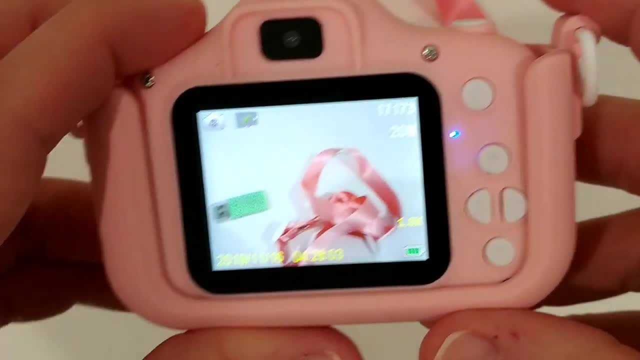 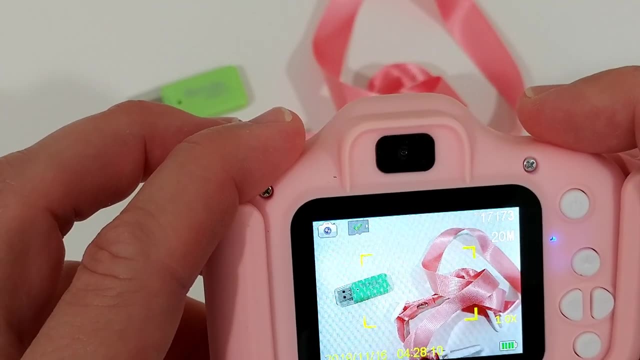 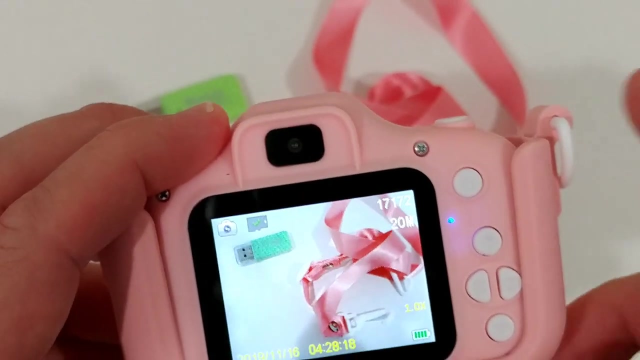 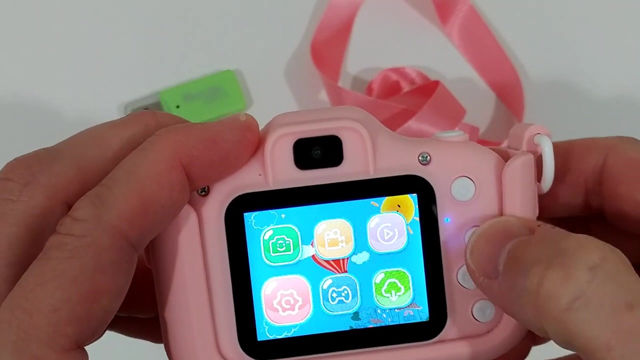 So you can see, it takes a little bit of time, but I have set it on the highest mode, 20 megapixel, which is probably too much, I would say. I mean, with this sensor and lens it probably doesn't make any sense to use 20 megapixel, So I'm going to use something in between now So you can see how this works. We go back to the settings. here We have the settings. Yeah, so we have clicked on the wrong button, So we 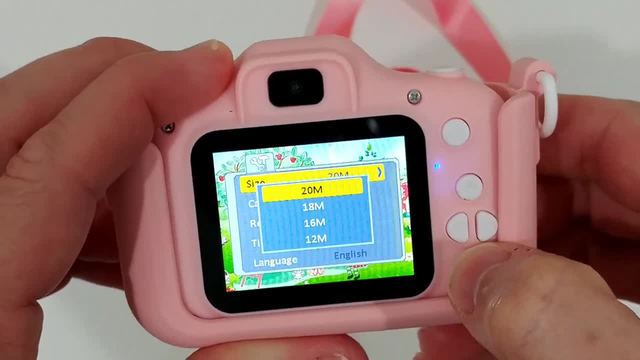 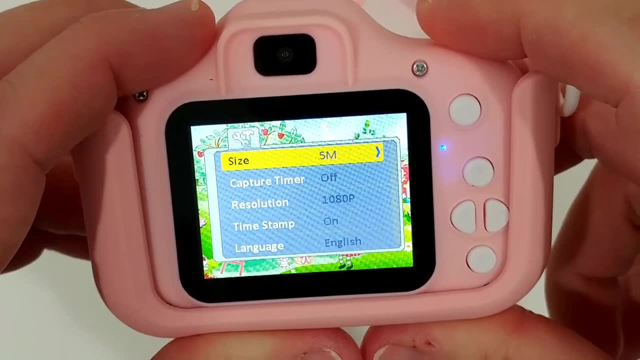 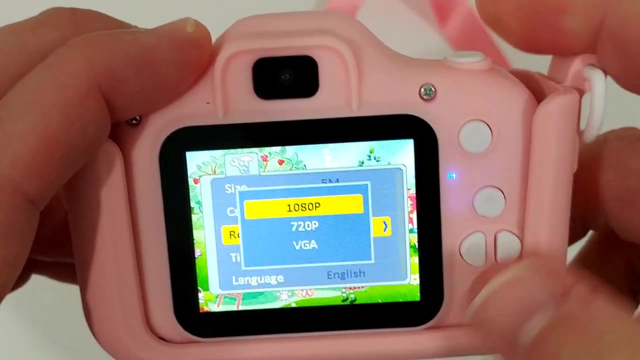 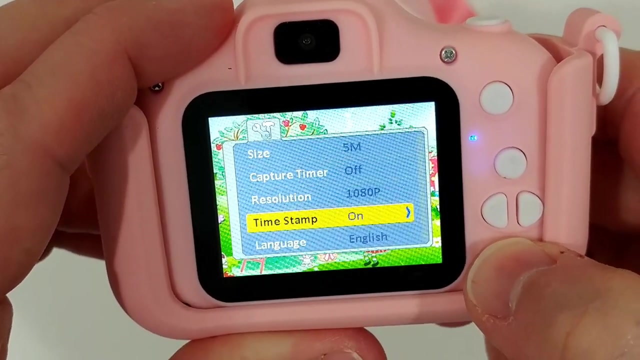 can choose the size. i'll go down a little bit. i mean doesn't make sense. maybe i'll use five megapixels. everything else doesn't make any sense. so you can see we have a lot of things like a timer. resolution for the video, vga 720p or 1080p. timestamp: you can select if you want to have it. 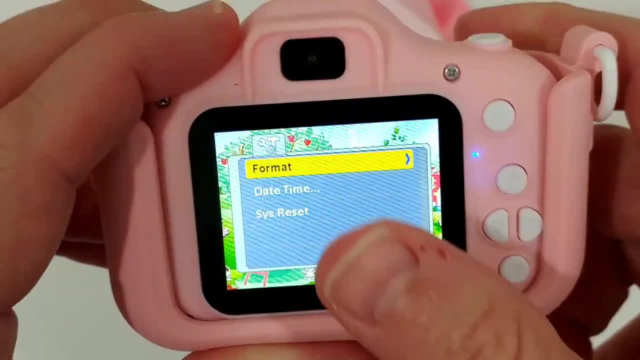 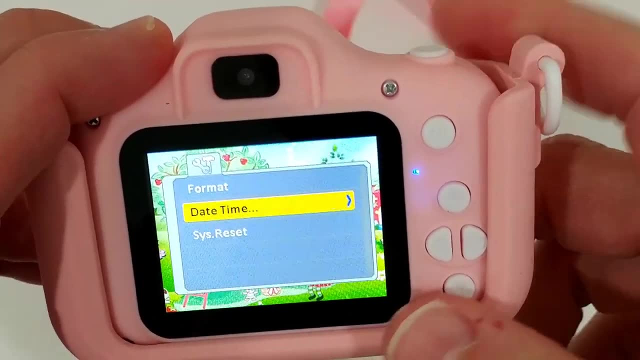 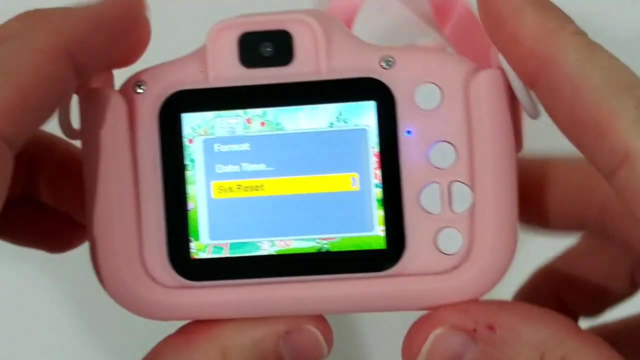 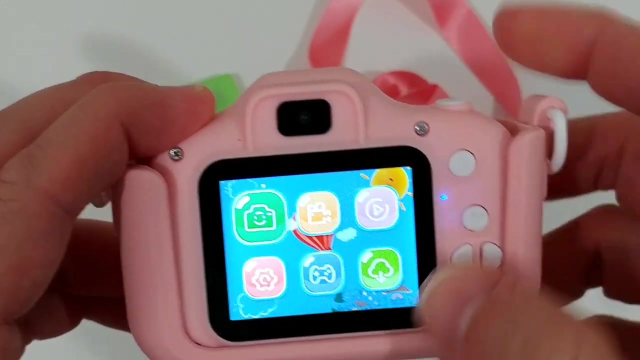 on the picture, language format, the sd card format and then the yet date time, which we can set here, and total system reset. we can also use this. there's a hole here. which we can use for total system reset is if something goes wrong, so let's go back and do another picture. 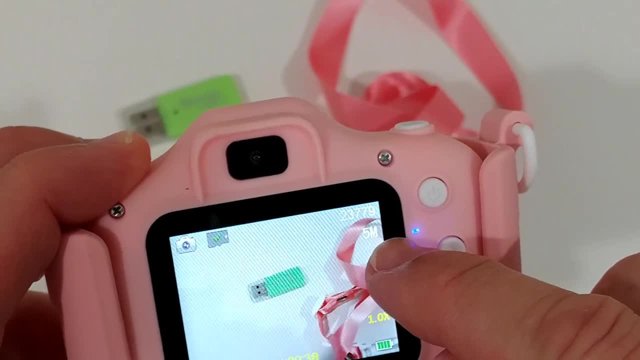 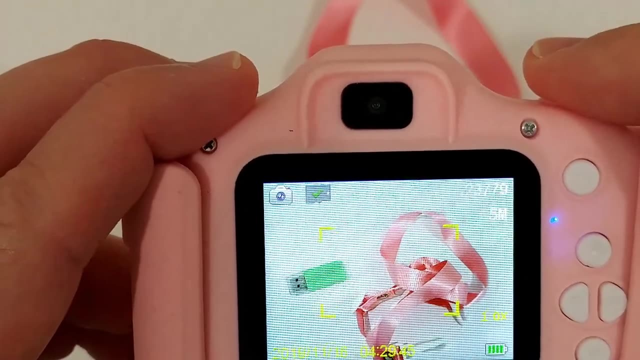 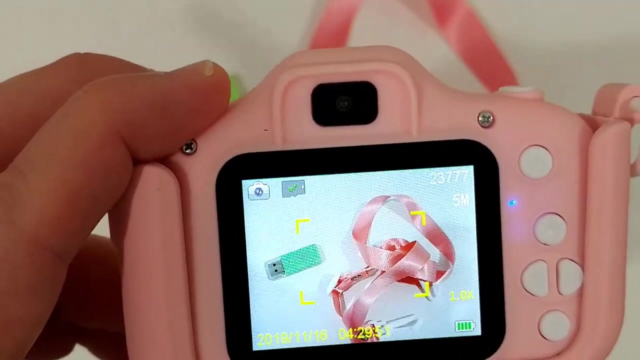 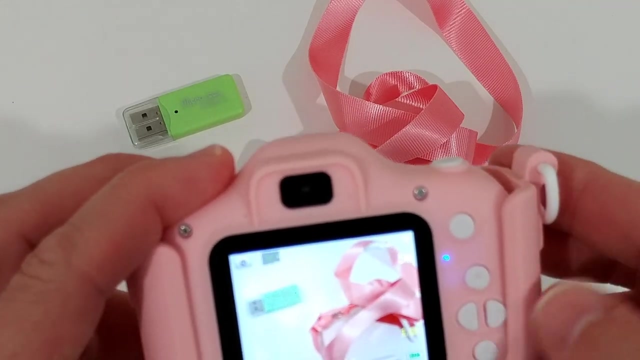 as you can see, now it's showing five megapixel here and we have 23 000 pictures left, so we can make pictures so till they are grown up. so you don't have to worry to buy additional uh storage cards or something like that. it will last forever. so that's the camera. let's go back to the video mode, so 1080p. 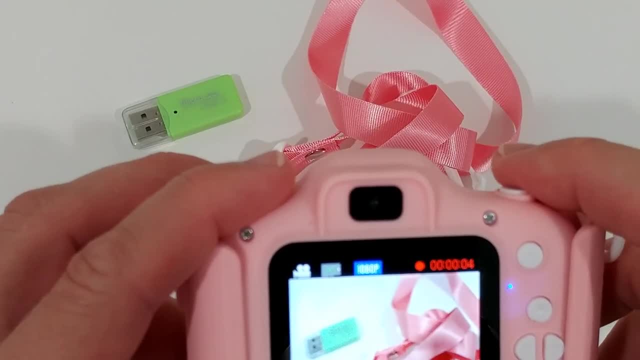 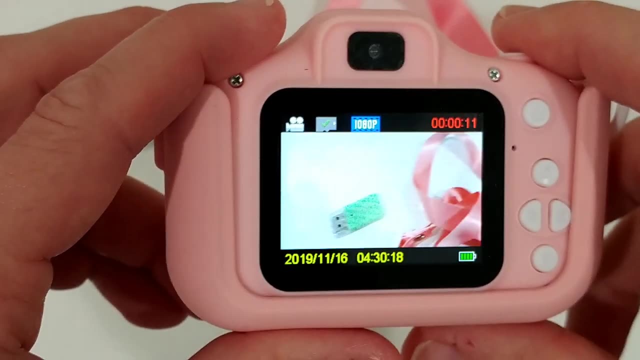 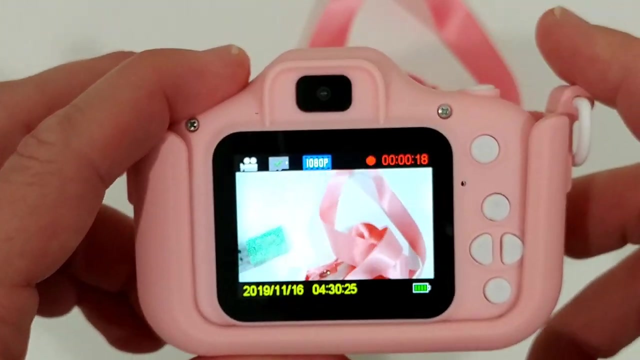 uh, it's. i think it should be with the microphone so we can hear the sound. it's not stabilized, so that's easy to see when we move the thing around. absolutely no stabilization. and i haven't found any stabilization in these settings, which is: yeah, it is as it is. i mean you. 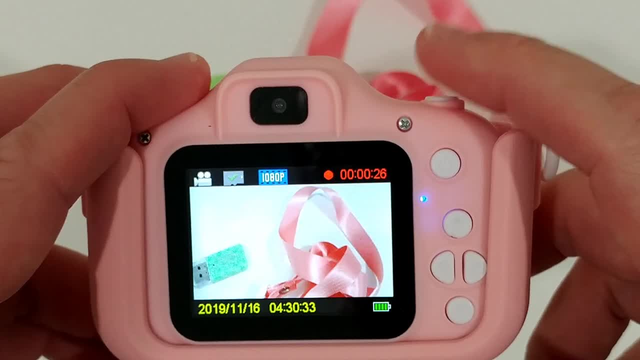 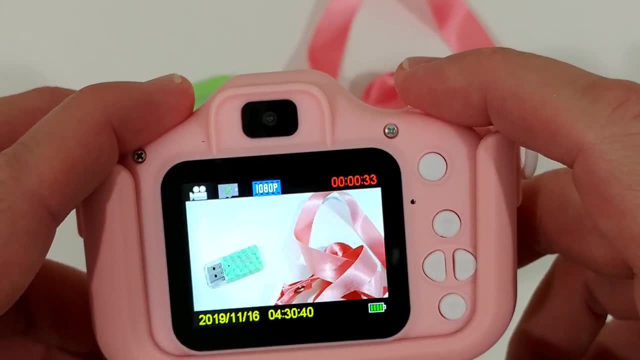 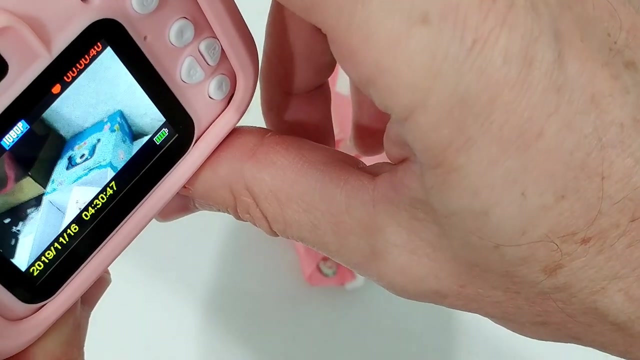 cannot expect everything for 32 dollars. would have been nice to have some kind of electronic image, but we can see that the image is not too bad, so it's not really a problem. we can see that the image is not too bad, but the picture at the moment looks not too bad. i'm pointing a little bit. 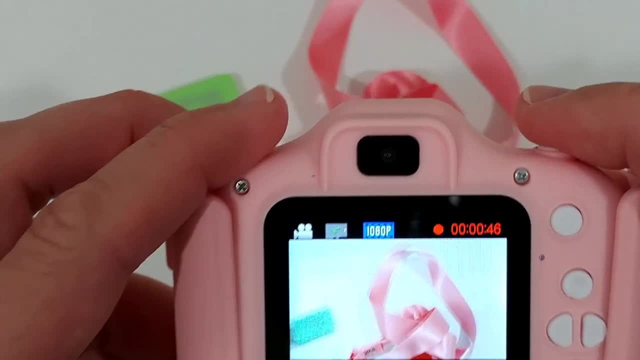 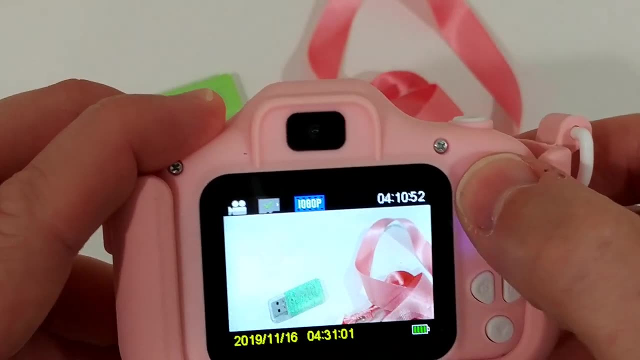 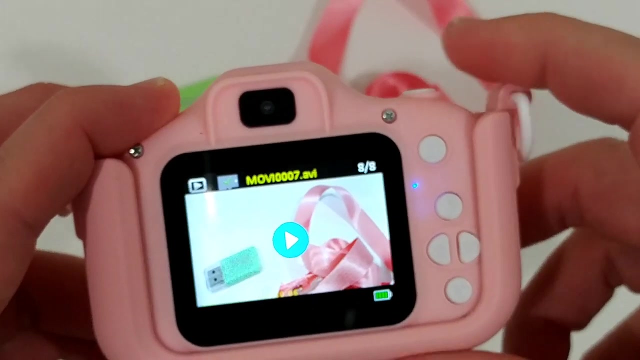 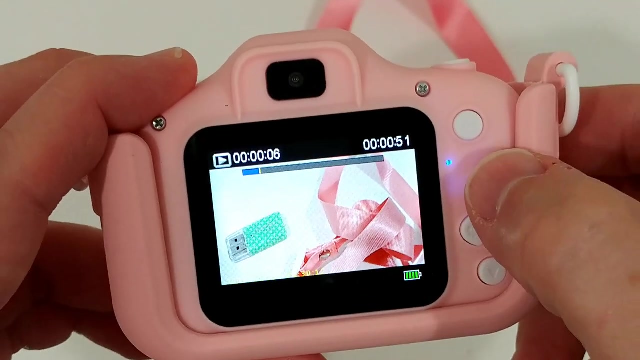 to the side here. maybe we get a better focus, but still, we can nicely focus, even close. i mean, focus is no focus it's, i think it's- a fixed focus. so we stopped recording that and let's go back. what to play? let's play this here. yeah, it's not very loud, maybe we can increase the. 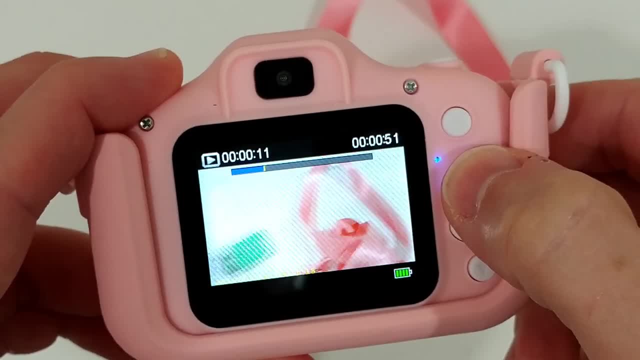 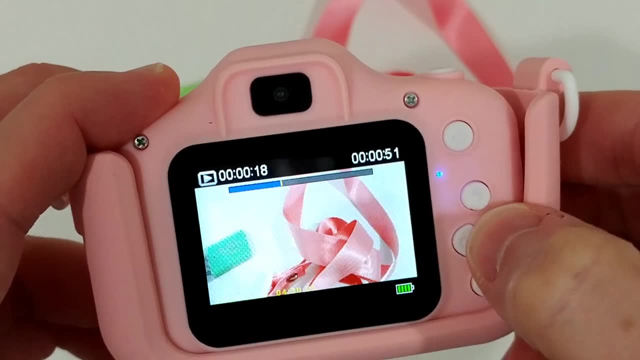 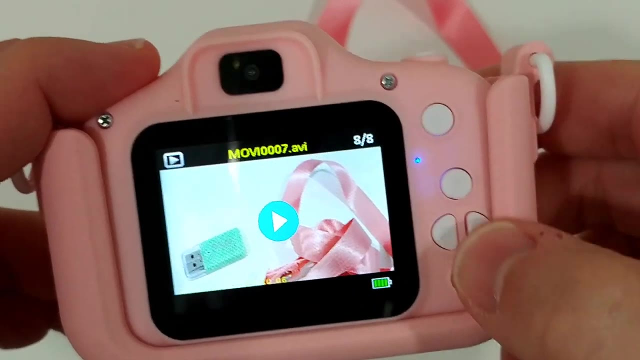 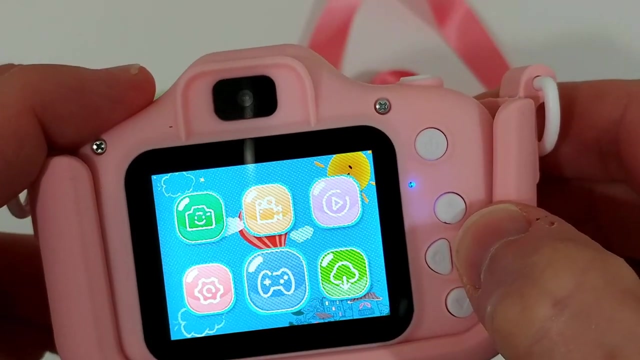 volume doesn't look like we can increase that here. can we go back and forth? I think there's not much we can do. we can just go back then to the menu or go to other footage. that works definitely good. yeah, we have already seen the settings and here we have games. yeah, we have any, even some games. you can confirm that? and 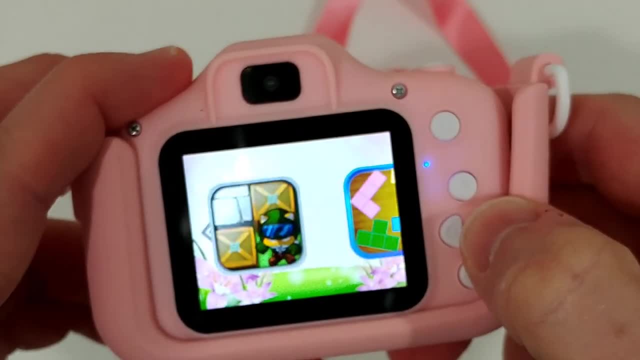 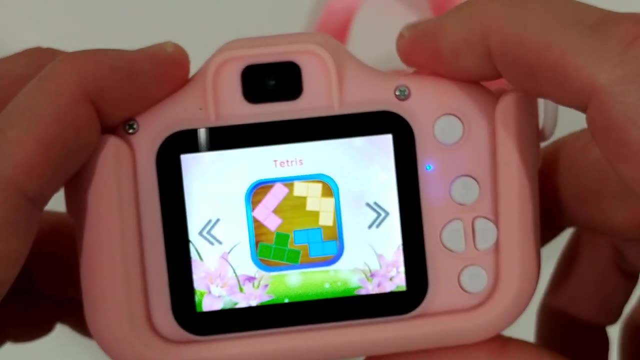 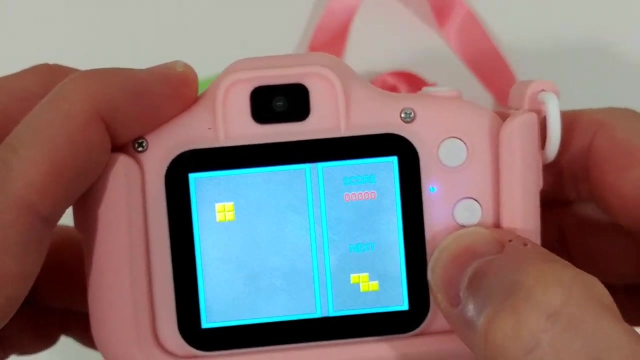 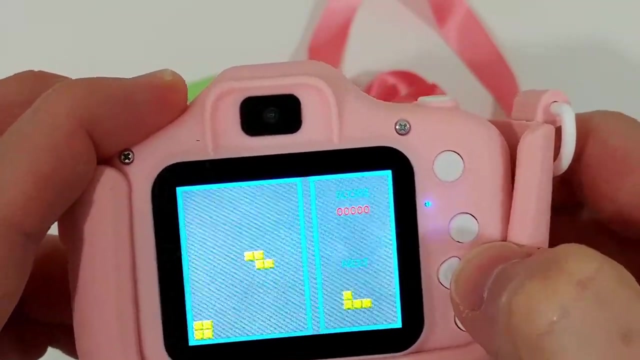 we have snake, we have Tetris, we have push box. yeah, three, basically three games. do they work? I mean, here we have the Tetris, let's start and see if we can do something. is that now let's switch? yeah, okay, I'm not the best Tetris gamer, definitely in. 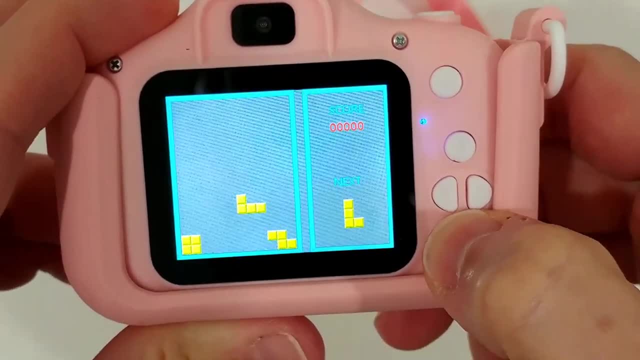 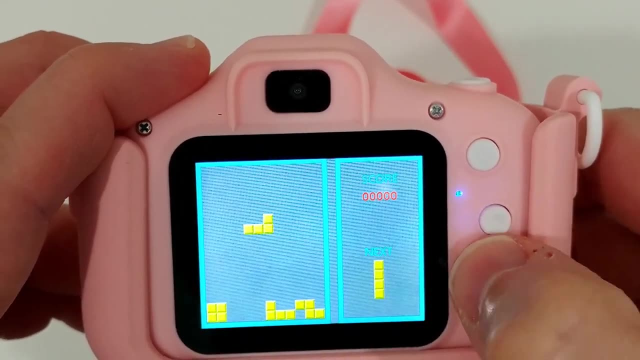 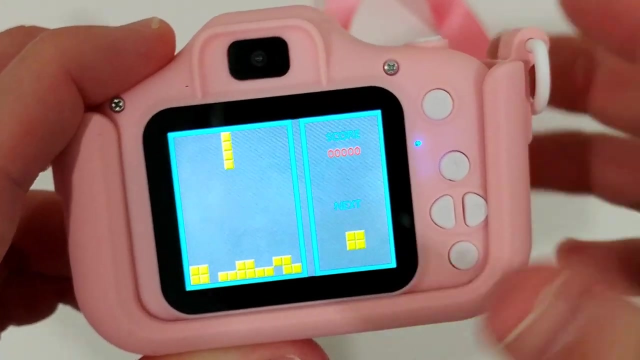 this world, but looks like it's definitely. yeah, I'll miss that button here, okay, but apart from that, I mean we can only turn it in one direction, how it as it looks like. but it's pretty cool for kids to have this, so you don't have to give them your cell phone all the time. 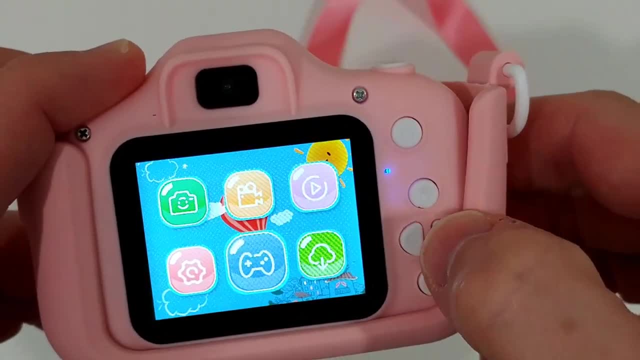 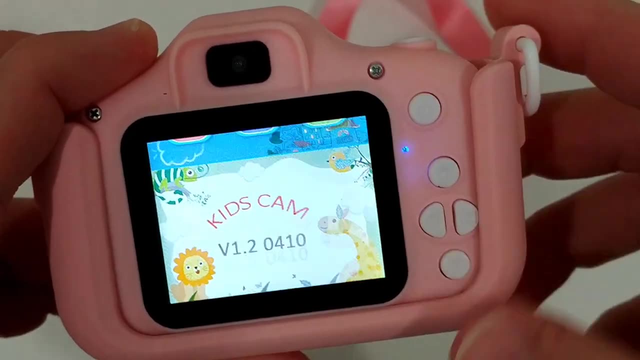 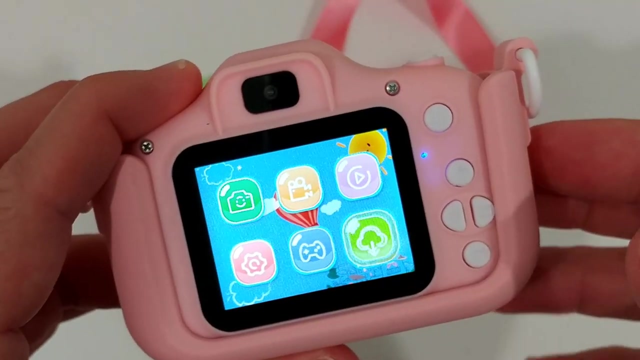 so let's go back. nice thing here. what do we have here? I think that's a firmware upgrade. at least it shows you the firmware, current firmware, and that's about it. and now I'm going, I am going to make a few pictures and I'm going to 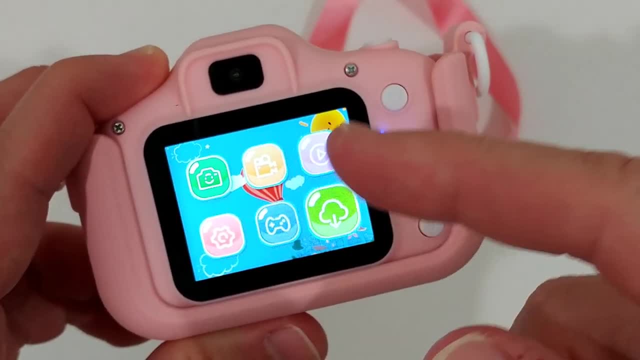 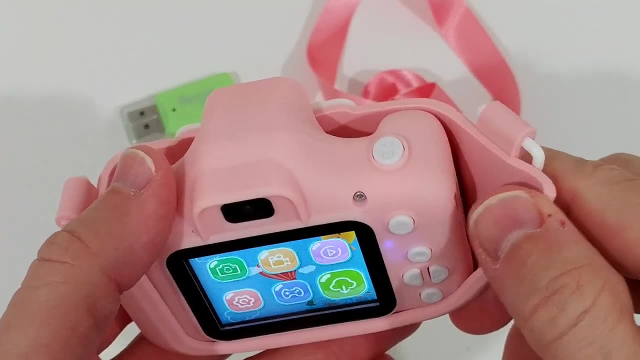 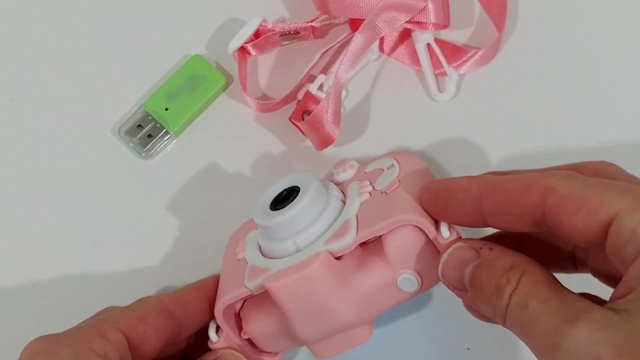 show you that in better resolution so you can see them better than all the other about it. but you know you can see that with a nice recording. so on the screen here. by the way, before we leave this thing here, I wanted to show you that I mean this outside, the outside semi case. that's soft plastic, it is a. 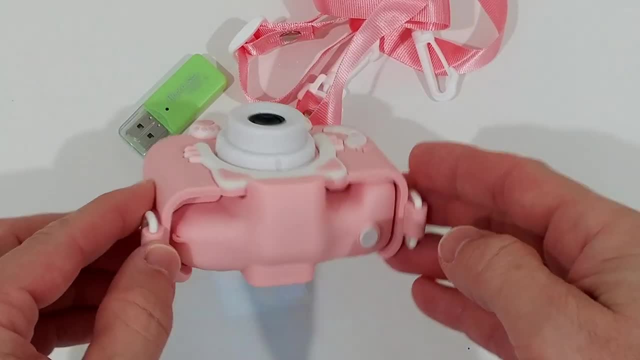 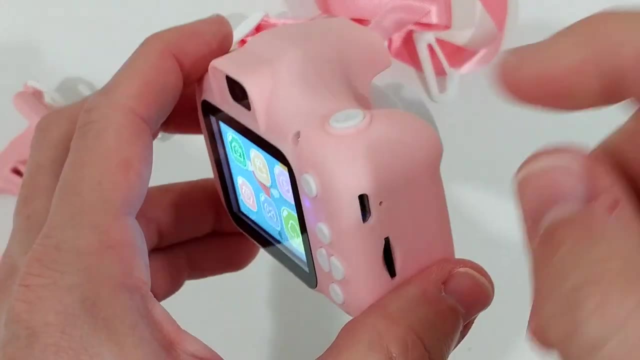 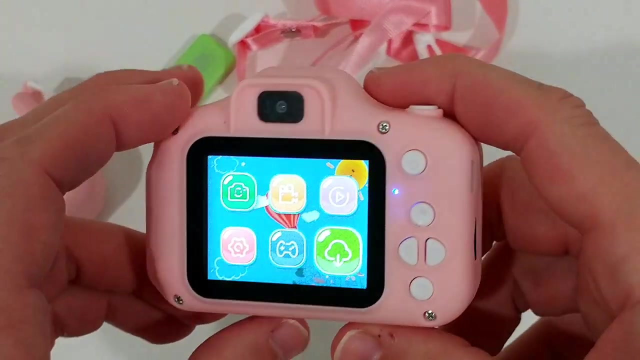 really nice protection. as you can hear here there's no hard sound when we take it out of the yeah semi case. here that's a yeah, rather hard case, so you can hear that. so it's not so good protected anymore, but i mean it's really super lightweight. i mean i don't 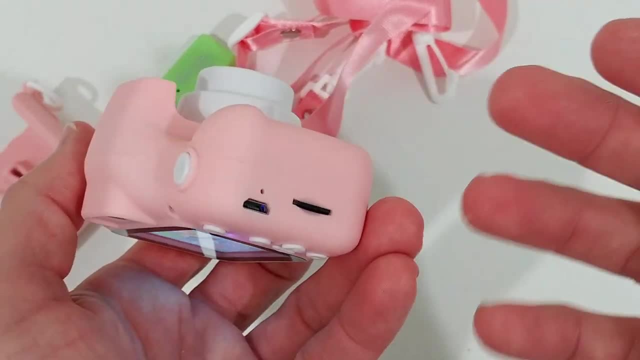 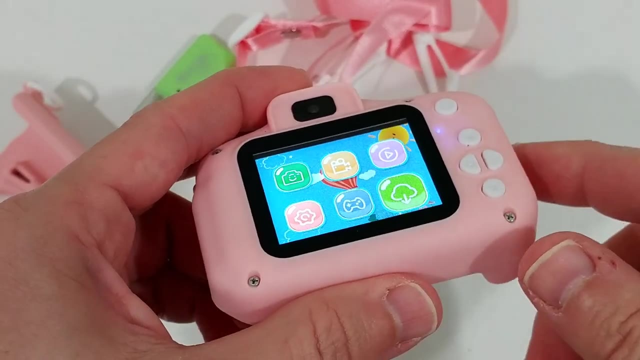 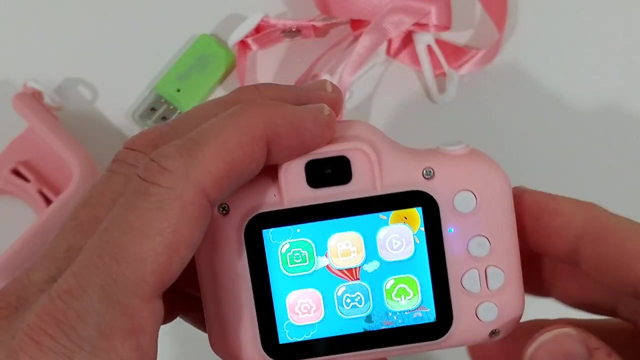 expect to fully break if we drop that. it's so lightweight and, yeah, plastic looks like really stable. the only thing was with the screen but it if it really falls out the screen protection, then you can add a few drops of instant glue and thing is done again for a couple of years i guess. 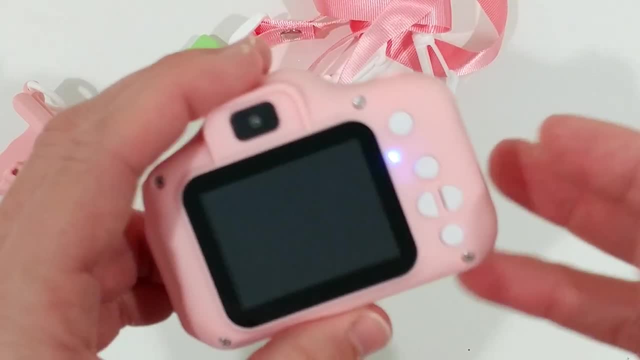 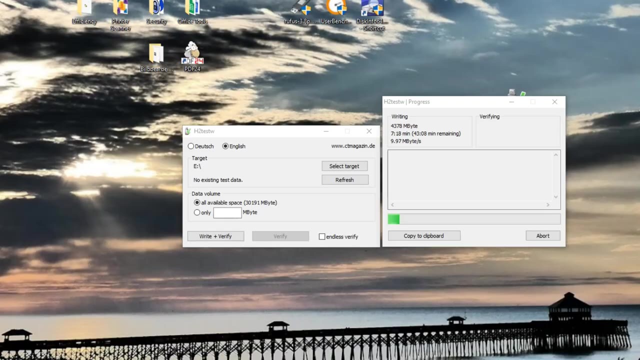 so we have even a screen saver which saves some battery- really nice. so, yeah, let's do the pictures and let's look at them. so till now, everything has been really really positive. i'm really positively surprised about everything. so till now, everything has been really really positive. i'm really positively surprised about everything. 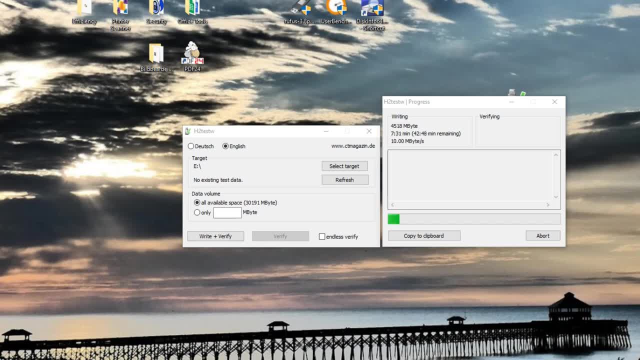 i mean how much stuff you get for 32 or- yeah, i mean they are always between, let's say, 30 or 40 dollars- how much you get in this price range with everything? i mean the packaging, the camera with the case and the strap and the storage card and even the cable, and, yeah, everything works right. 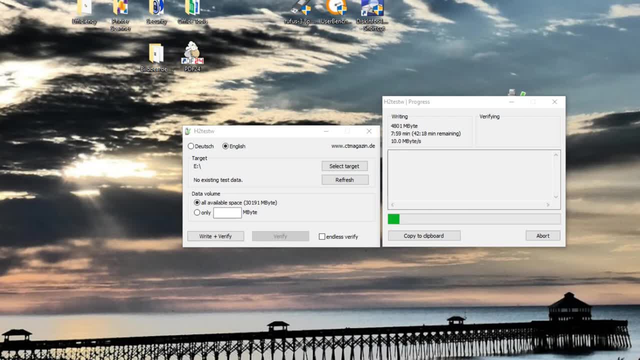 out of the box, no problem. i didn't have any errors or whatsoever. uh yeah, and the menus are really easy to handle. i mean, the menus are really made for children, i have to admit, and it usually it's really difficult with cheap chinese manufacturers. sometimes they create user interfaces which are really really super. 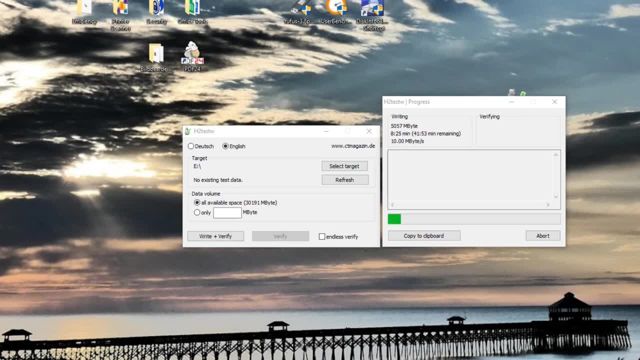 difficult. and with this one, i yeah, i mean, this is him, this is really something which you could give to. and with this one, i yeah, i mean, this is him. this is really something which you could give to, i think, small children to learn a little bit how about to interact. 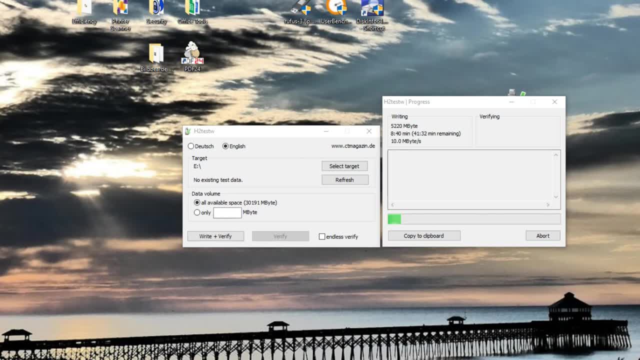 with electronics, and it even contains some games. so yeah, it's. it's a really positive surprise till now. but now let's go to the ugly part of this review. first thing, we have this micro sd card. i've put this in in the adapter stick and i'm testing it now with the 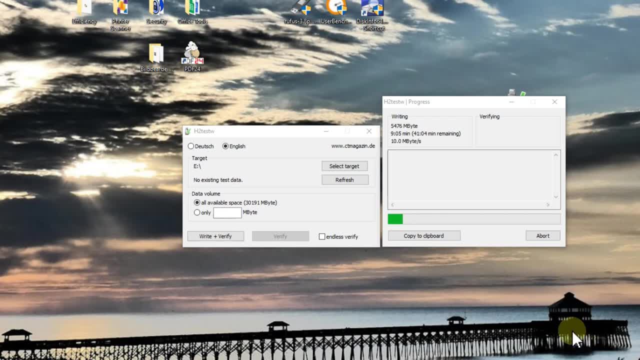 uh hardware tester to find out if we really got 32 gigabytes of storage. i mean, the worst thing would be if you give it to children and they make videos and pictures and at the end you will find out that storage was not 32 gigabytes but only maybe one gigabyte and it was overriding. 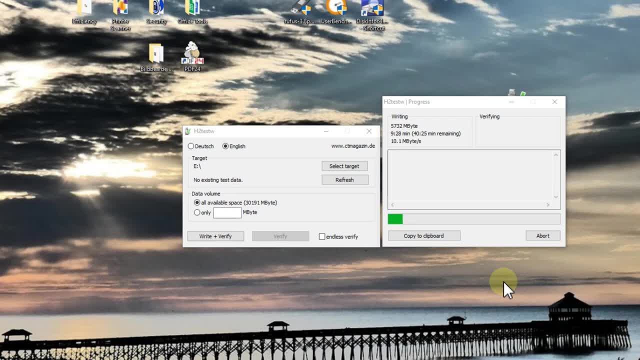 that happens a lot with such cheap micro sd cards. they say, yeah, they're have 32 gigabytes, 64 gigabytes, whatsoever, and at the end it turns out the storage is much smaller and it's just overriding old footage. that would be horrible and the worst and a total disaster. 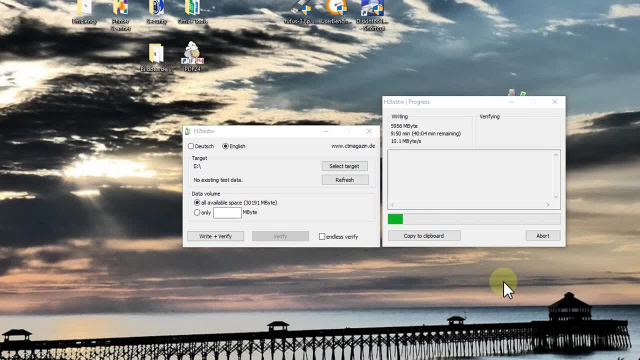 and absolute deal breaker, of course, for this thing. so, but i'm still testing it. as you can see, it takes quite some time and i will definitely let you know, either at the video or or i will put it down in the description or into the feedback area, so we'll know. 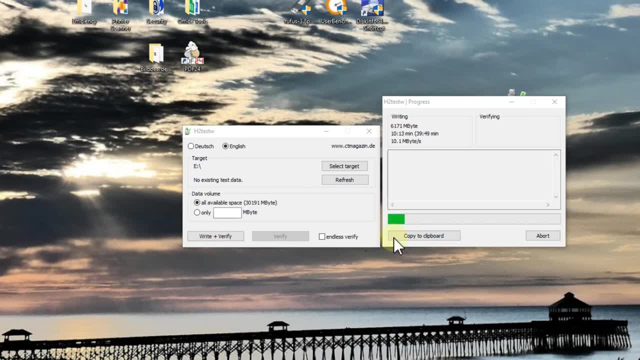 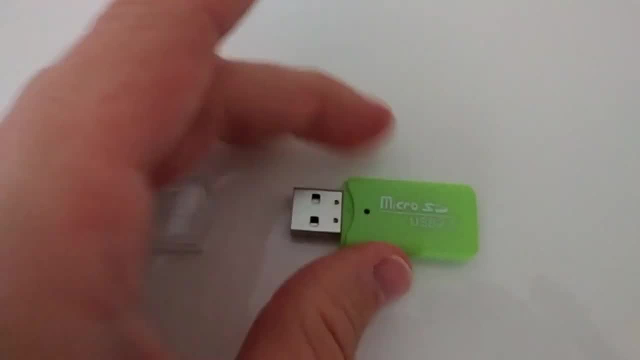 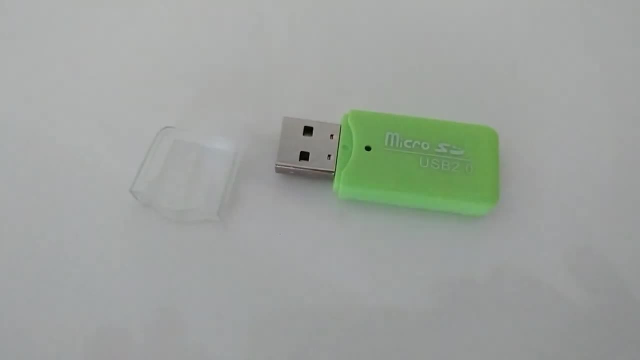 uh, yeah, so you will know at the end if the micro sd card really works or not. yeah, two more things before i'm going to show you the pictures. here we have the usb reader with the micro usb slot in the back. i've been trying to transmit the picture with this one. it worked really well. 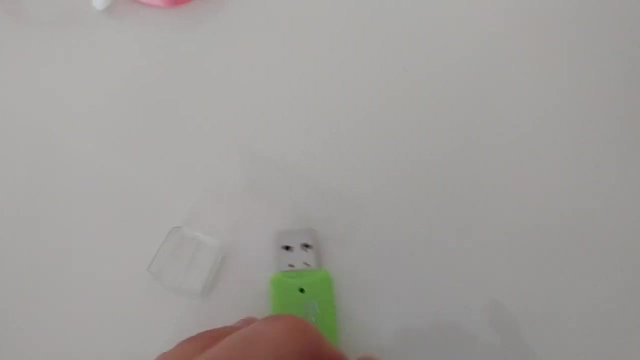 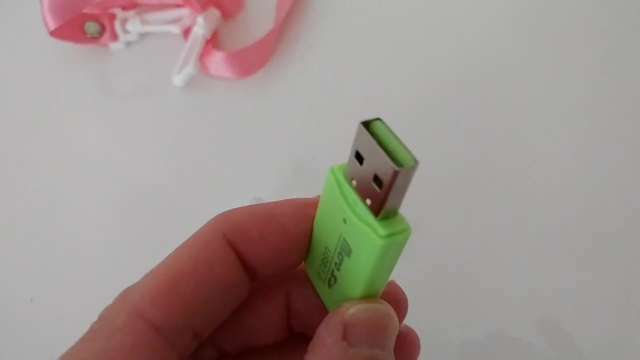 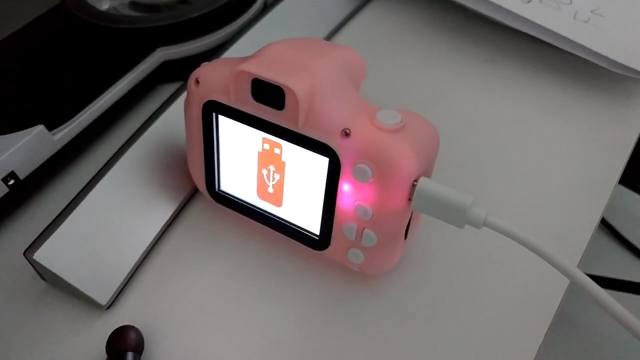 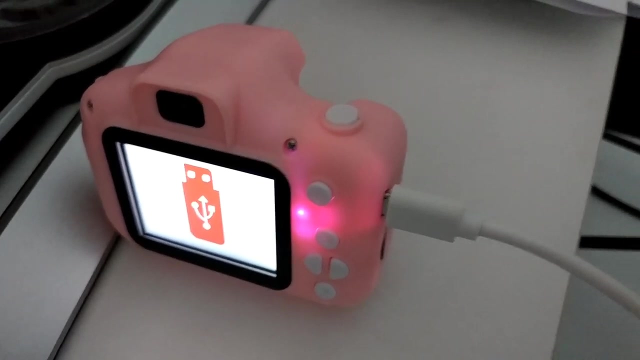 i did have to to plug it directly into my computer. when i plugged it into a usb hub it didn't work. so i highly recommend to use it directly in your computer, and same thing with the camera itself. so it's definitely possible to connect the camera with the pc with the micro usb. 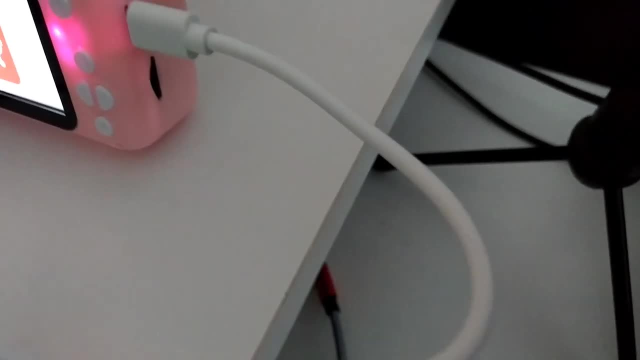 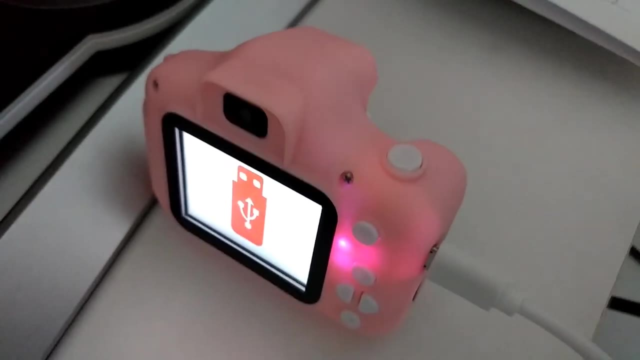 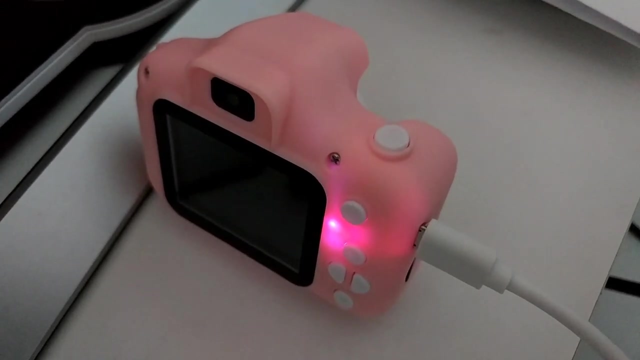 cable here. but you have to plug the end other end of the cable direct directly into your computer and not using a hub, otherwise it could be that you can't read your photos. so at least in my case it it was like this that the the pc didn't, didn't recognize the. 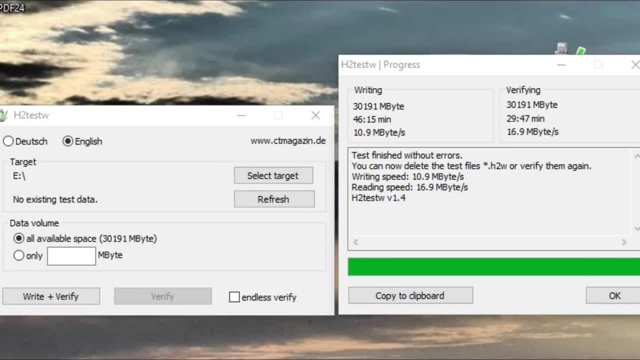 camera. so here i have my final results from the micro sd card and the test was finished without errors. and you, here you have the writing and reading speed and i mean that definitely means that we get a full 32 gigabytes micro sd card which is working, reliable and at least that's. 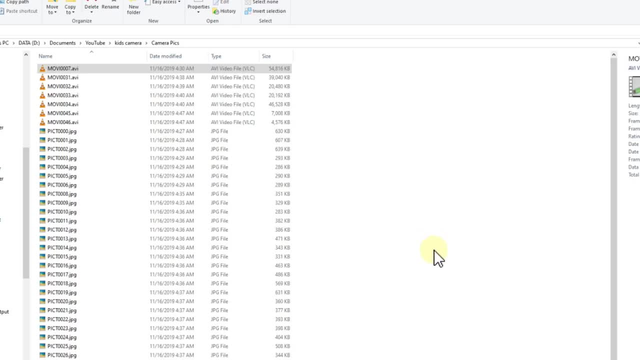 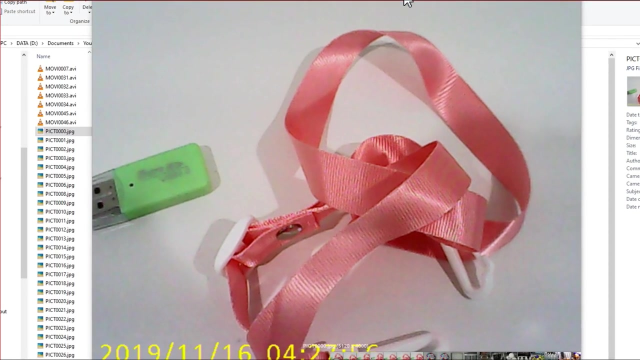 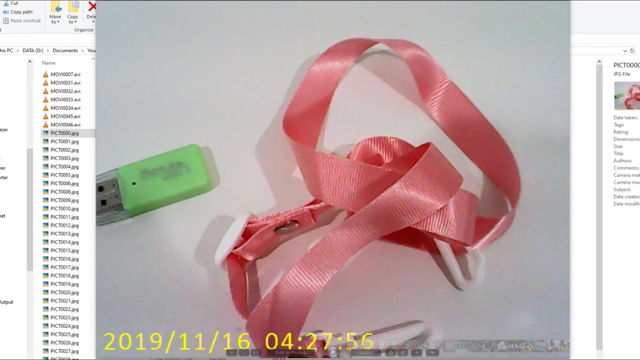 uh, definitely a positive thing. but even apart from that, i have really bad news for you, and the bad news is really the footage. so let's start with a few pictures here. i hope they will open more or less nicely. i will adjust these sides. no, i think it's about: yeah, a little bit, let's make this a little bit bigger. so, as you can see, 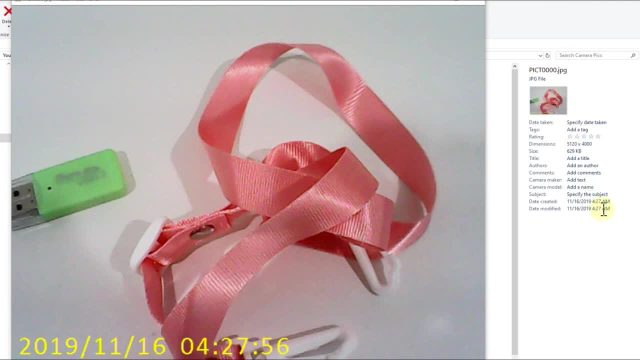 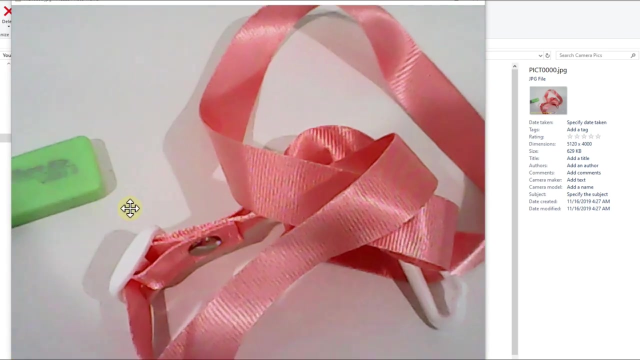 yeah, even on the right side you can see the resolution. so i here i had a 20 megapixel picture, so they're really made out of the thing. a 20 megapixel image i mean at the end it's maybe a 720 or something like that. it's absolutely nonsense to store the. 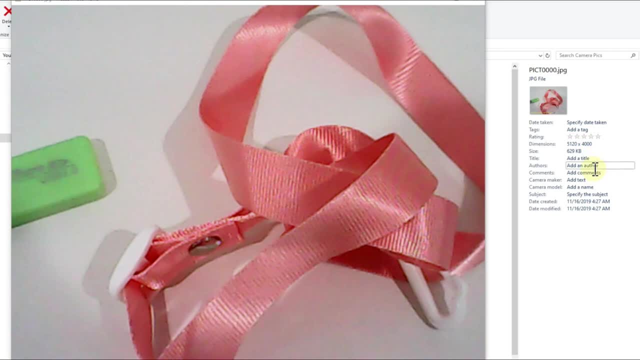 things in 20 megapixel size. i mean, of course they will be compressed down. the effective size is only 629 kilobytes, so you don't have to fear that it will fill up your computer. but still, it's absolutely no sense to interpolate this to 20 megapixels. 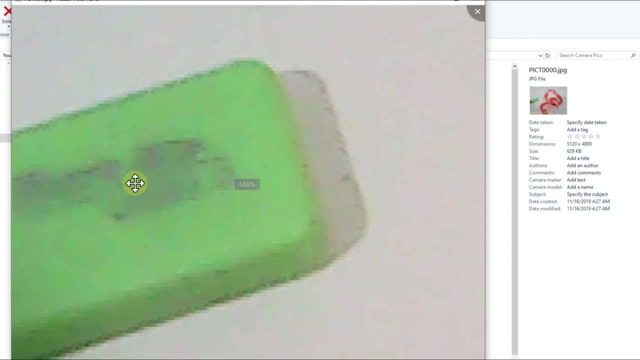 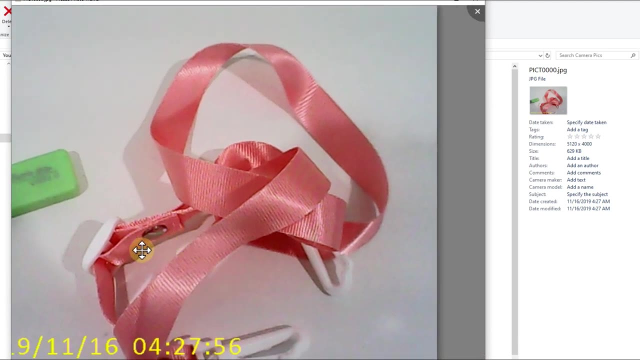 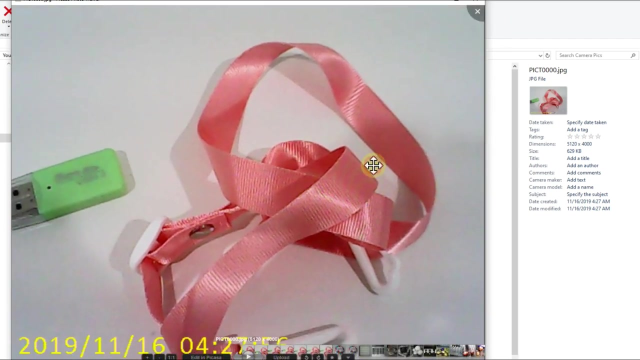 so when you have results like this, you cannot even read a text or something like that. the only sharp thing is the date and time, which is only thing. apart from that, it's totally blurry, washed out whatsoever, so really close to a complete disaster. i mean, we have nice colors, but that's. 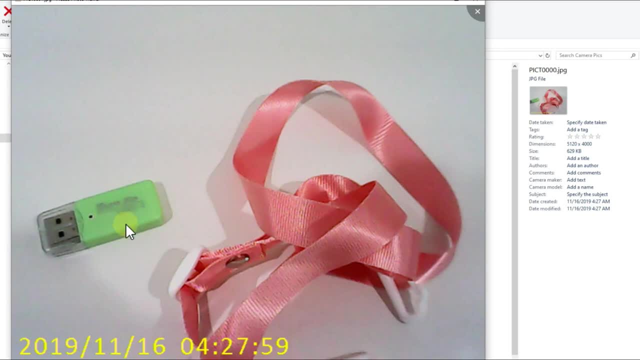 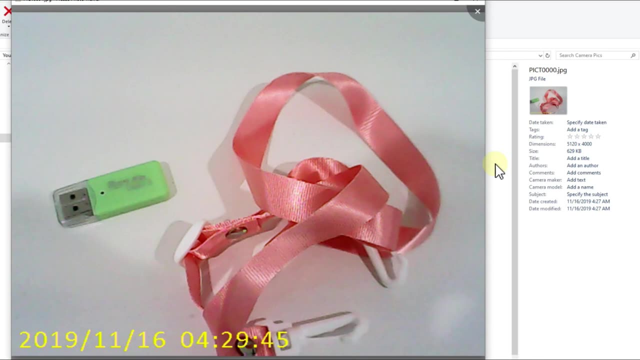 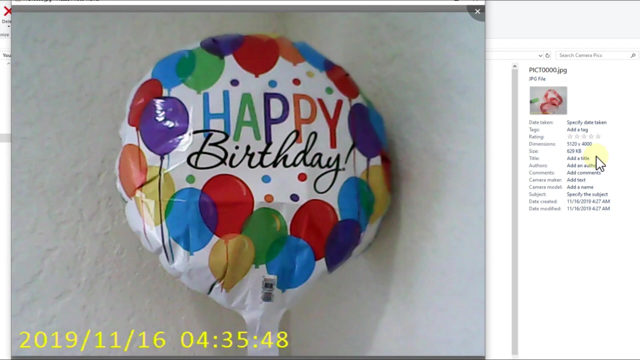 about it. there's nothing to read here. i think there is something written, but you cannot read that. let's go quickly through the images. still 20 megapixel here. yeah, it looks like they have made everything in 20 megapixel, even when i went down to 5 megapixel. 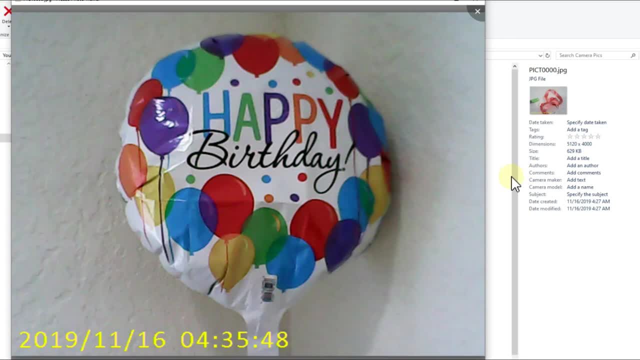 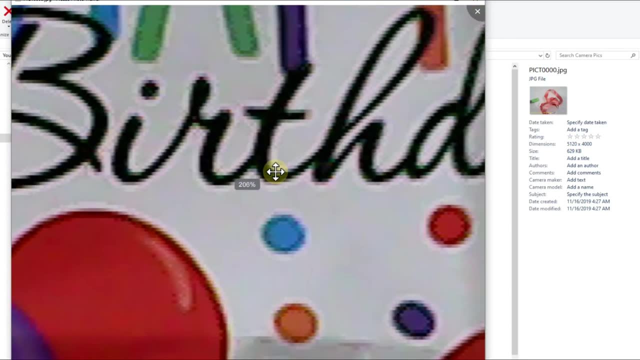 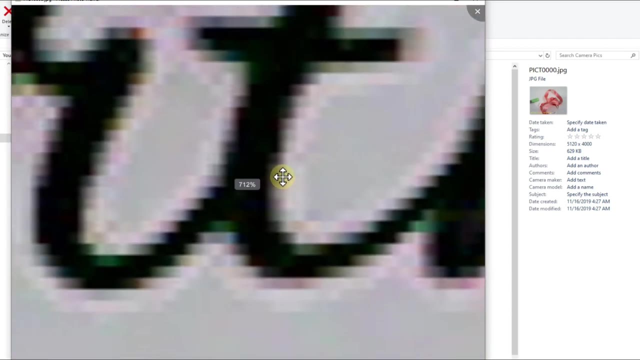 that's a surprise, so maybe it didn't store that. i have no clue. so here we have one image which is actually, yeah, that's almost the best what you can get, but you still see, when you get a little bit go a little bit closer, i mean it's totally artifacts, blurry whatsoever. um, yeah, i mean at. 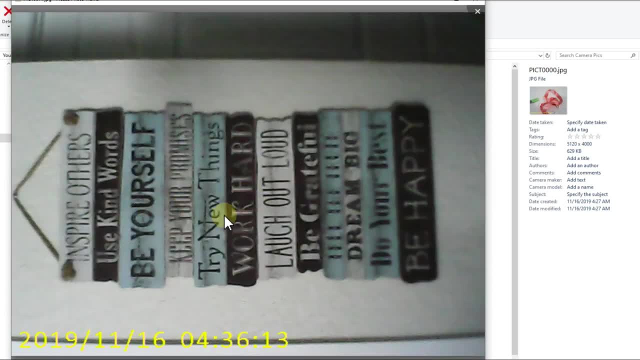 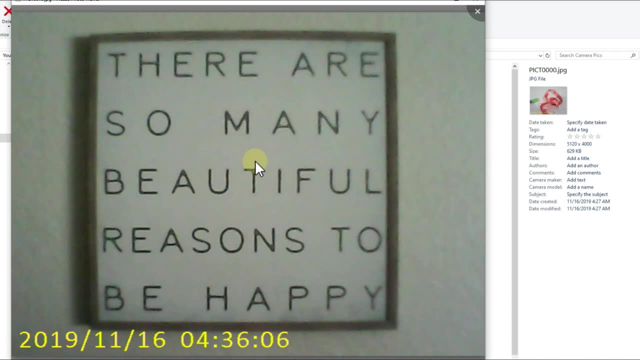 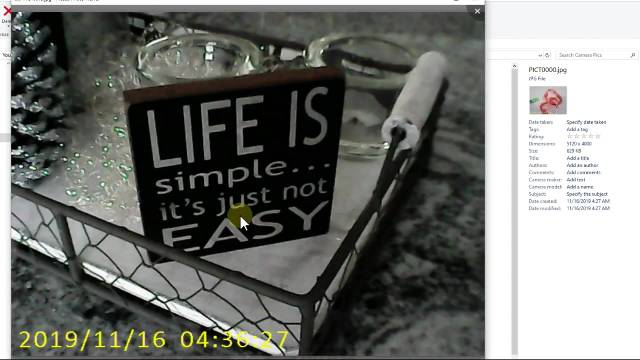 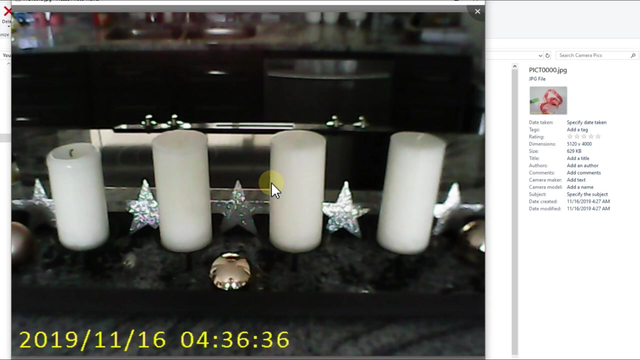 least this you can read here. i have taken this 90 degrees. it's hard to read. that's probably the best image here which i have made. overall. that's a candle. even hard to read these big letters. yeah, i mean, is it? is it really useful? i mean, these pictures can be really, really disappointing. the focus is: 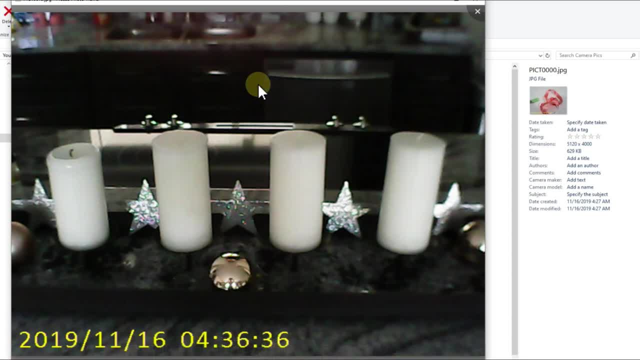 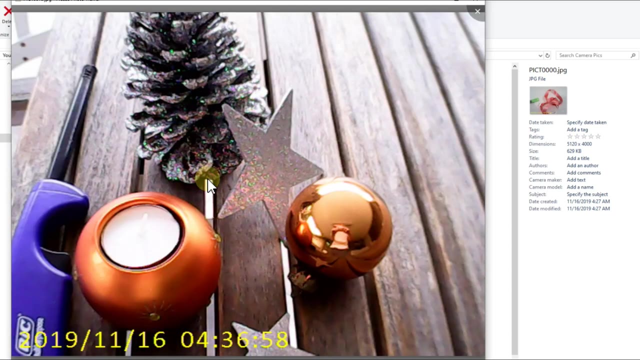 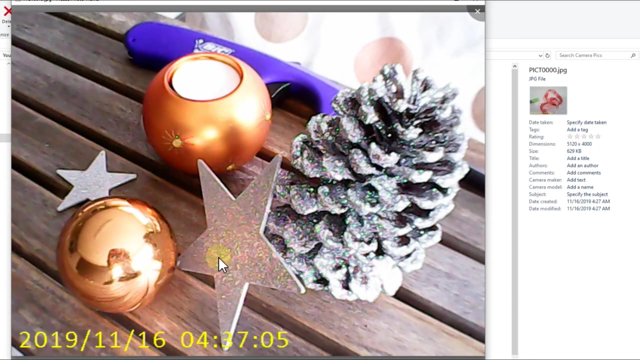 seems to be pretty close. everything far away here is even worse. i mean, i have to admit, here inside there was absolutely no light, it was overcast. there was definitely not much light inside, but still, yeah, i mean the pictures. this is outside, but even outside with enough light, it's even there really hard to find anything in focus. 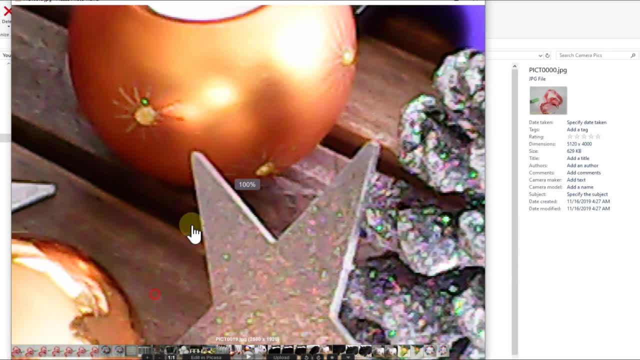 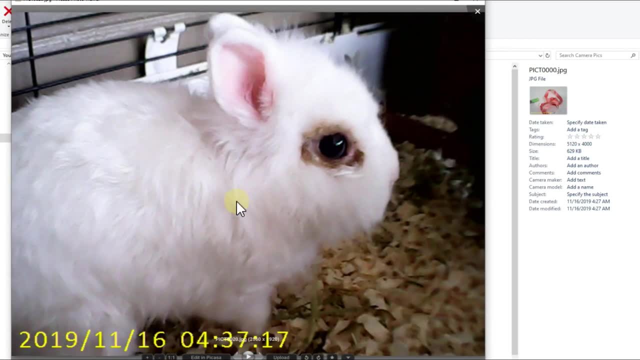 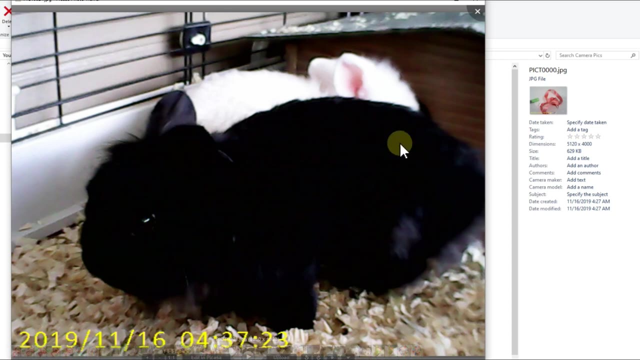 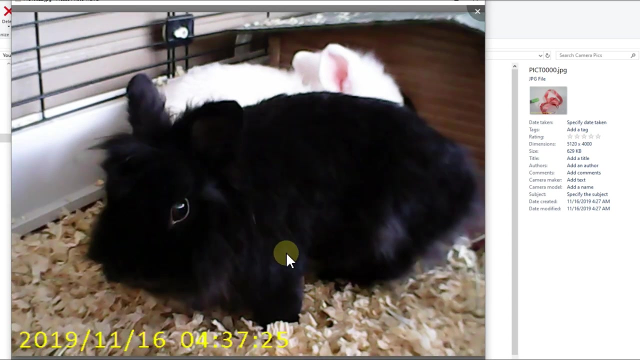 you can see all these artifacts. i mean, yeah, that's, that's really a bummer. i've been trying with the rabbit. i mean you can see it's a rabbit, definitely. but here the black. you can see there's just one black bubble here. i mean no hair visible, nothing, it's just just black. yeah, here a little. 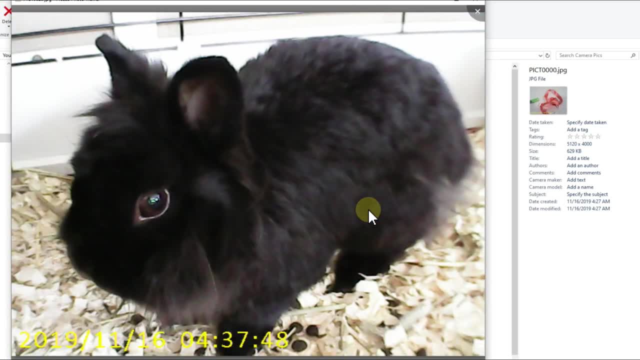 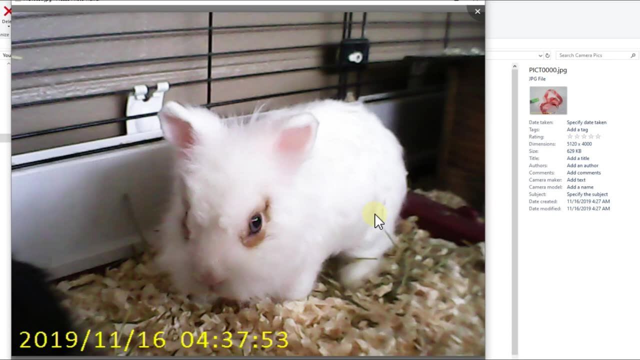 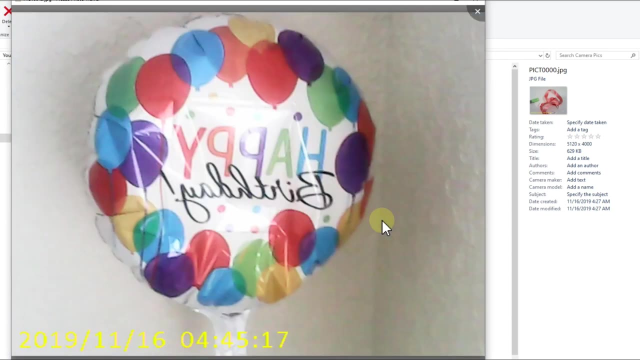 bit of the fur, but it's, it's really hard. i mean, yeah, it is disappointing. i mean, if you give it to a three years old, okay, yeah, maybe most of them, most of the pictures, they will just watch, probably on the camera, but you still want to have them, some memories later on. 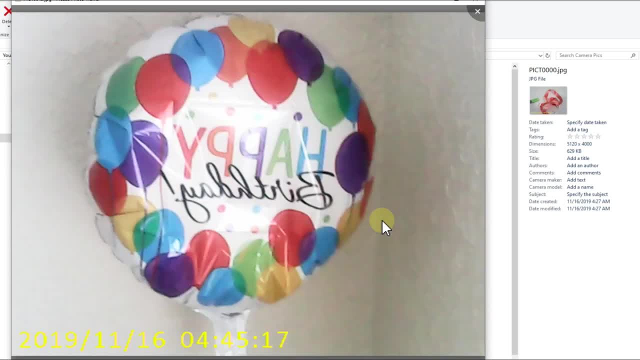 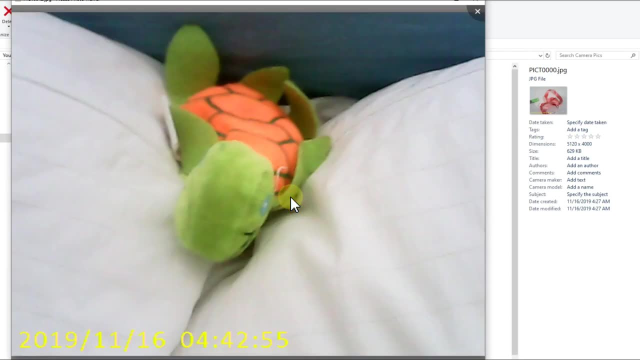 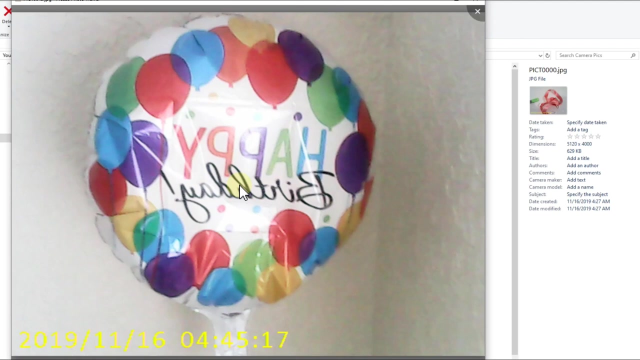 and when they watch at them. yeah, it could be pretty disappointing. uh, here i've made some selfies. yeah, here's the first selfie that's some kind of turtle and the balloon. i mean, this image of the balloon has been made with the selfie. uh, yeah, the camera, which is actually 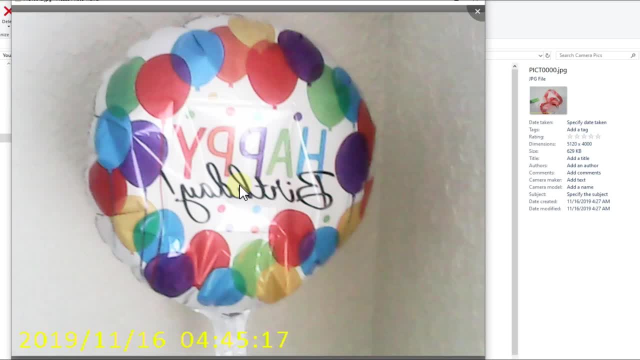 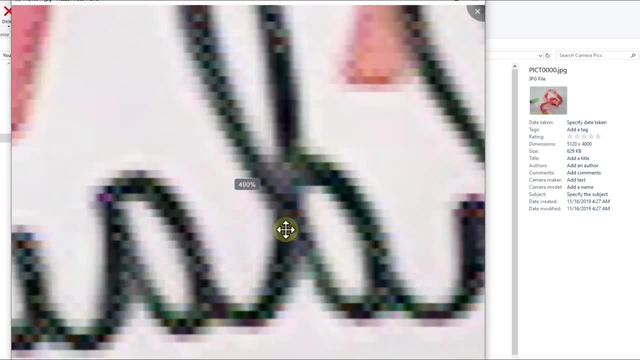 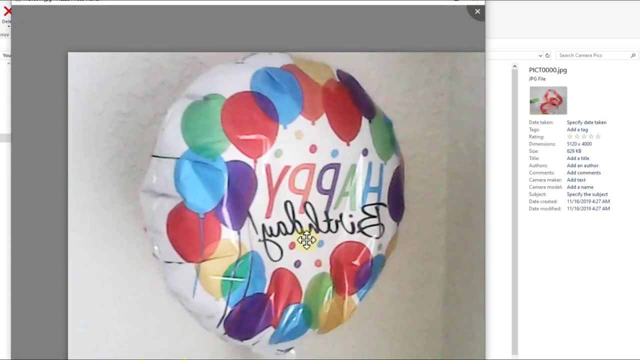 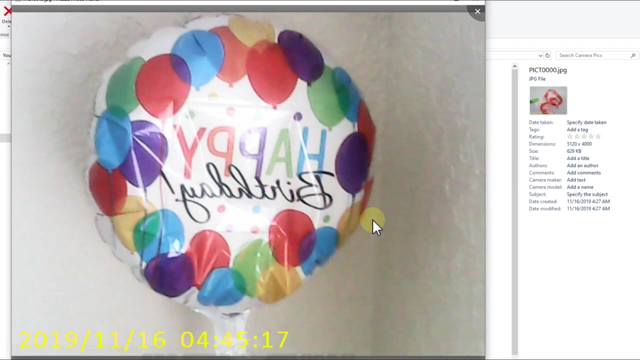 in the viewfinder just reverted, so you can see it's not much of a difference about same bad quality or even worse than the camera in the front. so yeah, pretty, pretty disappointing all the images, and they are all on 20 megapixel, but uh, it's a disaster. yeah, at least close to a disaster. 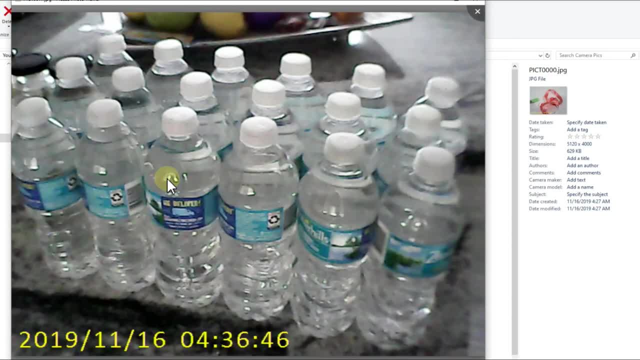 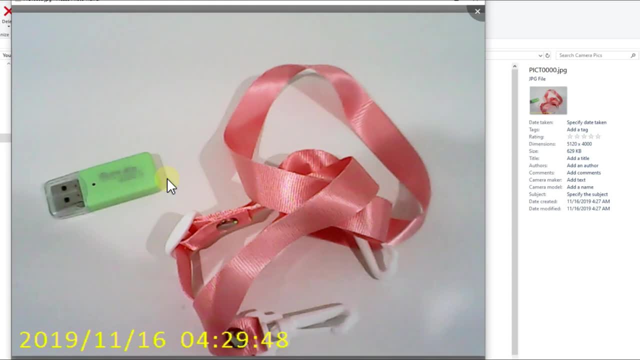 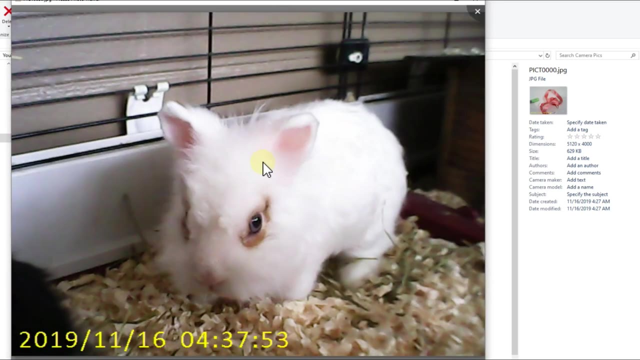 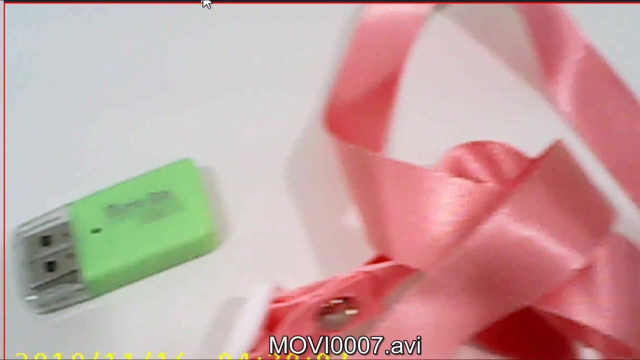 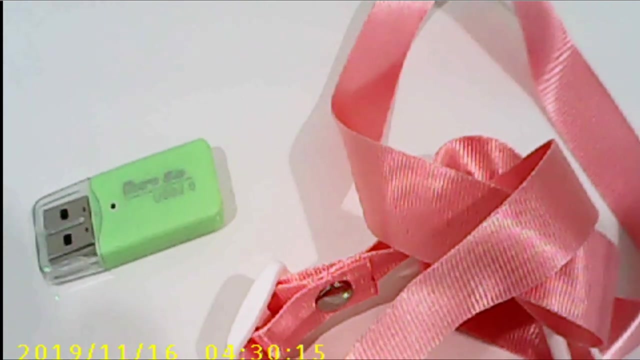 i was really excited when i saw the first images on the camera screen, but here, yeah, not really much positive to see. i mean, it was not really bright, not even outside, but still now let's try with the videos. so here you can even hear the sound. well, at least i hope you can hear the sound. uh, i stopped this for a moment. yeah, i just 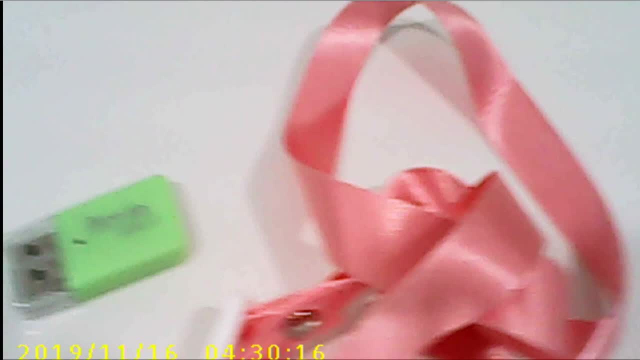 set up the system new and i'm not sure if you can really hear the sound, but the sound is horrible. you barely hear the voices and there's some really disturbing sound, like background sound. even even if it was not here in the room, it must come from the camera. it's similar to what some kind of 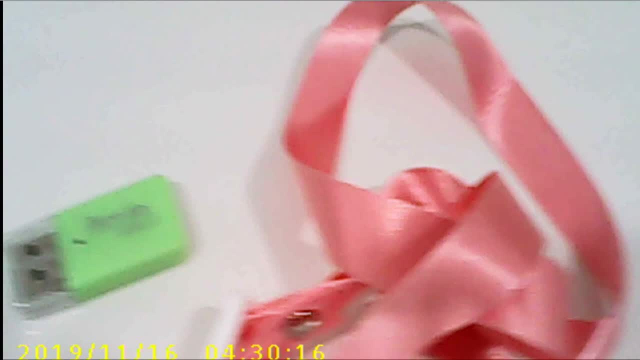 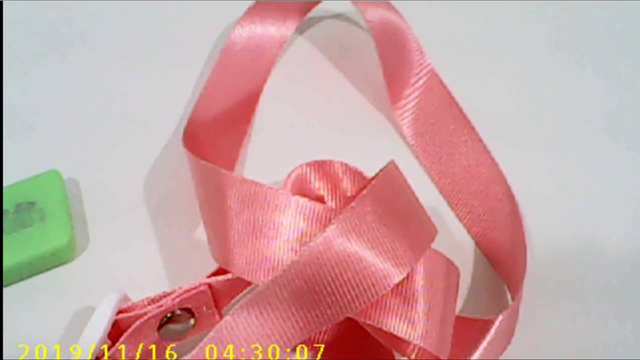 security cameras have this really strange sound like waves. uh yeah, when a boat uh rides fast on top of waves or something like that, it's really annoying. and i'm playing it again, maybe you can hear. so here we are. i think it should be with the microphone so you can hear. 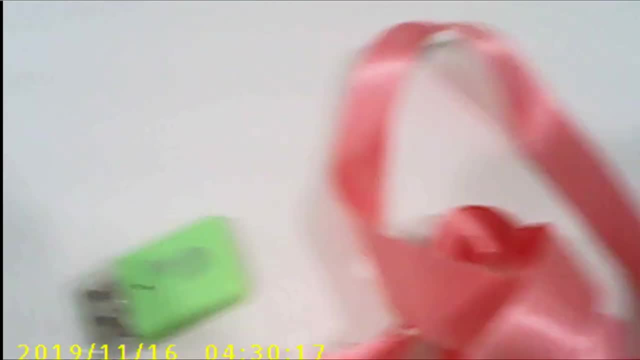 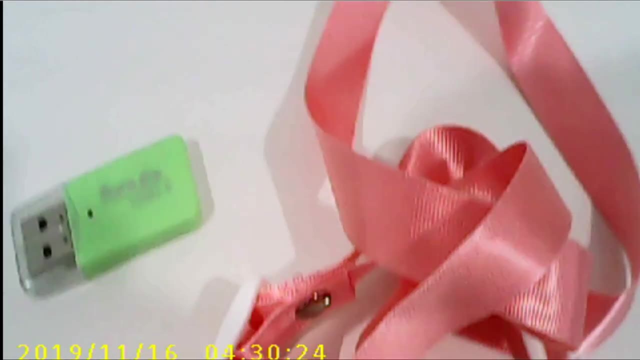 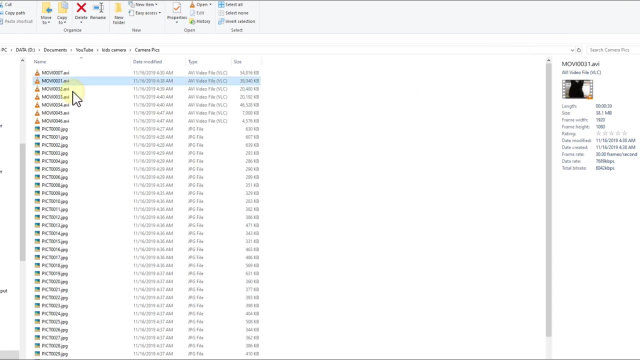 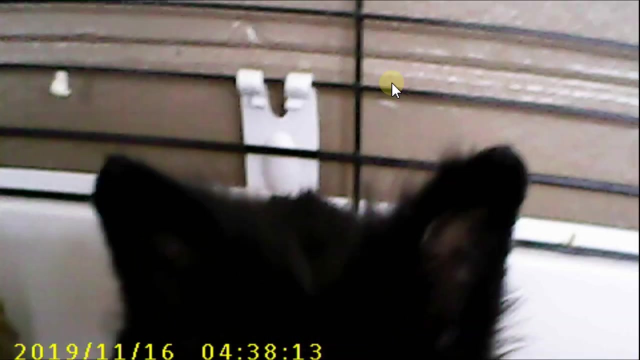 the sounds, uh, it's not stabilized, so that's easy to see and you move the thing around. absolutely no stabilization. and i haven't found any stabilization in the. i hope you have been able to hear that. at least you have been able to watch the video here. same thing, exactly same bad background. 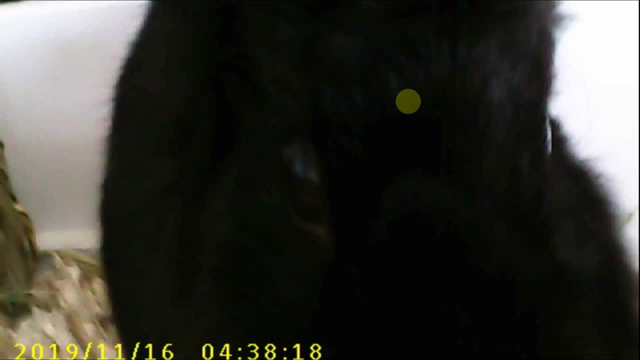 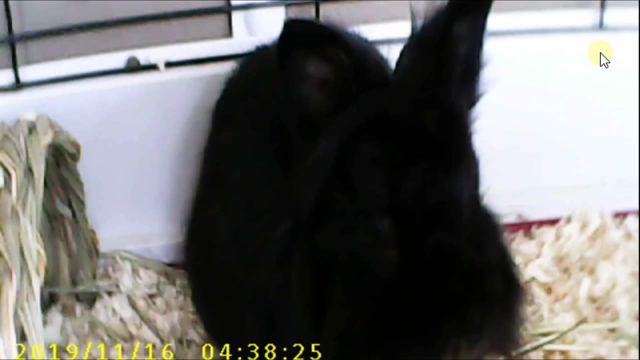 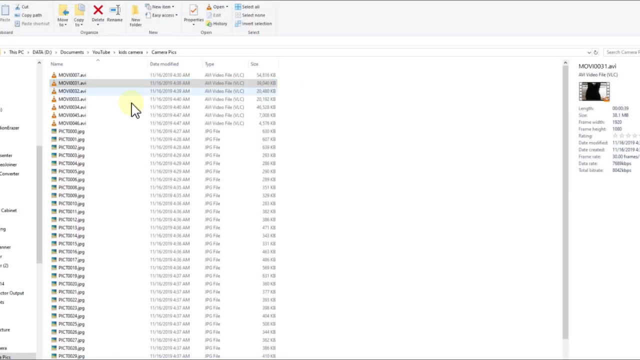 noise and everything, totally blurred, washed out. that's, uh, supposed to be 1080p. i i'm not checking that. i guess it's 1080p, but um, yeah, it doesn't help. i mean, the quality is absolutely a disaster. yeah, we, we can see. you can see that if you go to the details that it's showing 1080p. but i mean it. 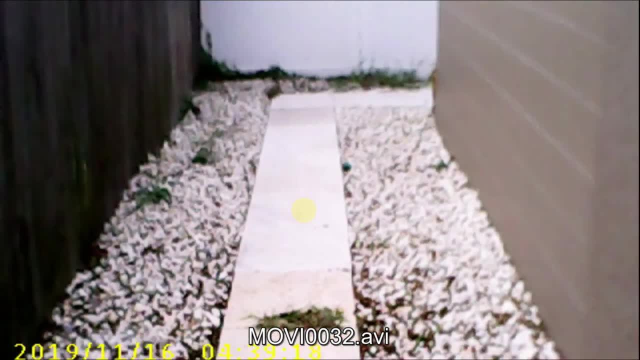 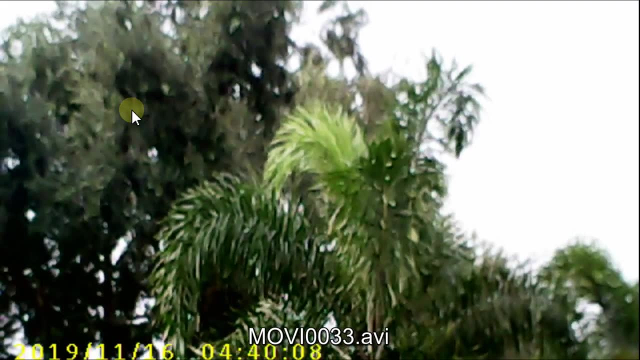 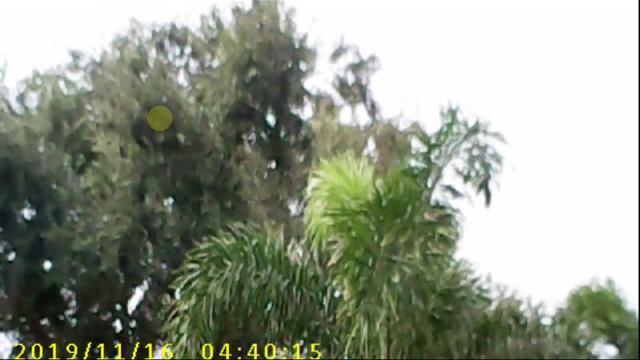 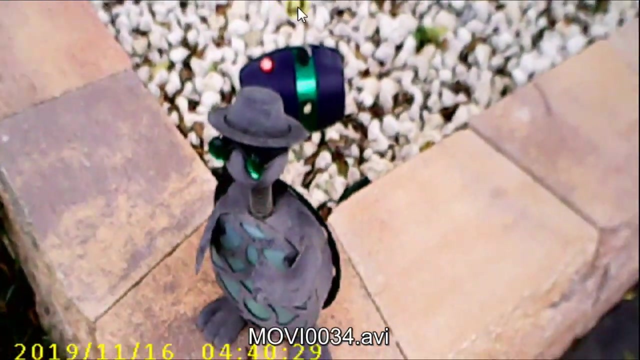 doesn't make any sense. that was outside, walking and having the camera in front of me. absolute disaster here. another thing: i was just standing, still just pointing at the tree- uh, in the wind, so it's barely visible that it's a tree. the end of the thing. produce the clicking. 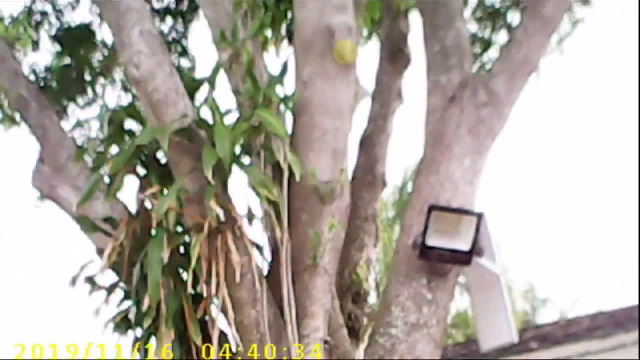 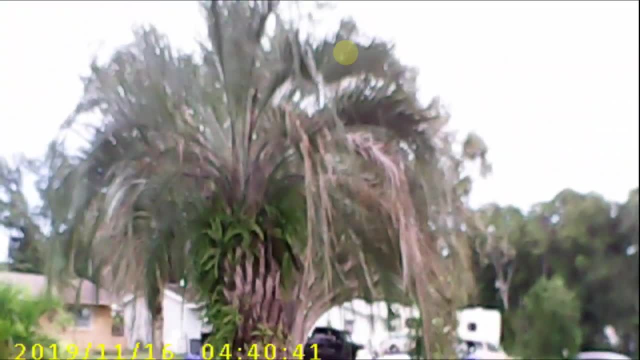 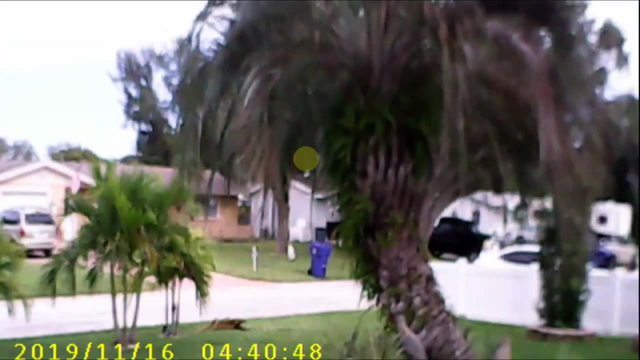 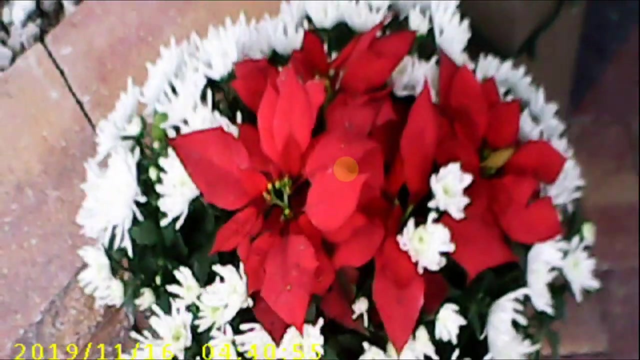 noise here a little bit moving around with the camera. so it is definitely a disaster if you have perfect bright weather and you keep your camera uh, focused, i mean, yeah, pointed at one location, yeah, you can see some things, but uh, yeah, it's, it's, it's, it's horrible, i mean, and there's something else with. 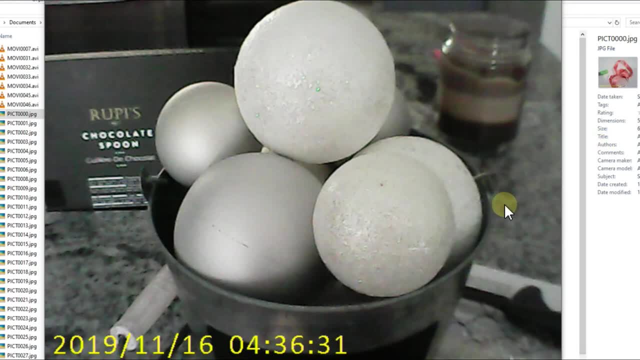 the pictures, something which you probably can't see on these images. it is the field of view. i've been testing the field of view and i would guess that it has about a 40 degree viewing angle. so i mean the gopro, we know they have about 100 and they can't remember exactly 120. 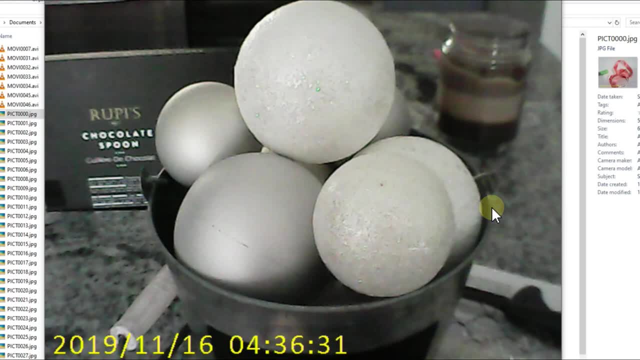 degrees, definitely not 160, 70 or something like that which a lot of cheap chinese camera action camera manufacturers claim. no one of these have 160- 170 degrees. most of them are around 80- 90 degrees. the gopro has about around 120 degrees. uh, good, cell phones, yeah, about maybe 80, 90, the widest. 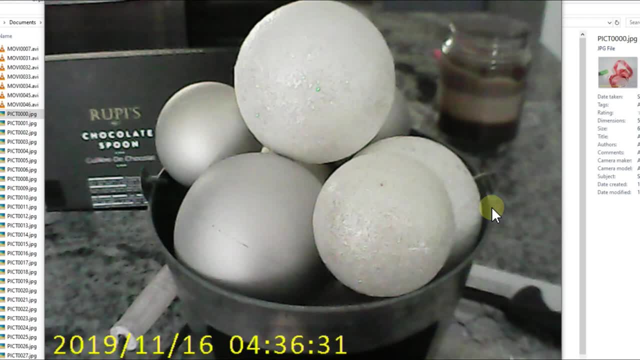 120 degrees. this one here has about 40 degrees viewing angle. a 40 degrees viewing angle- yeah, that's about it. it is as it is. you have to know that, don't even know, can't even remember what they write in the listing, if they have a wide viewing angle or whatsoever. 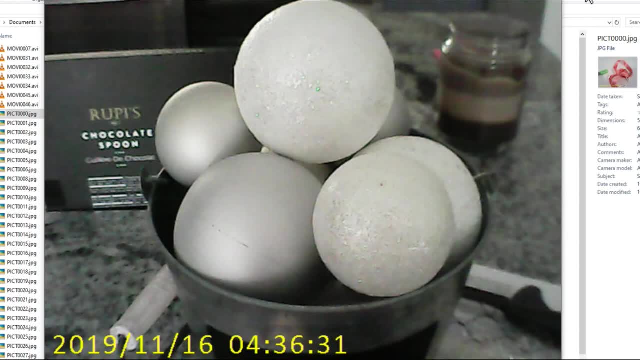 it's only 40 degrees. i mean you can work with a 40 degree viewing angles angle. yeah, of course there's quite some limitation and a wider field of view would have been nice, but um, yeah, even with this quality probably wouldn't have helped much. so that's me my final resume of this whole thing. i 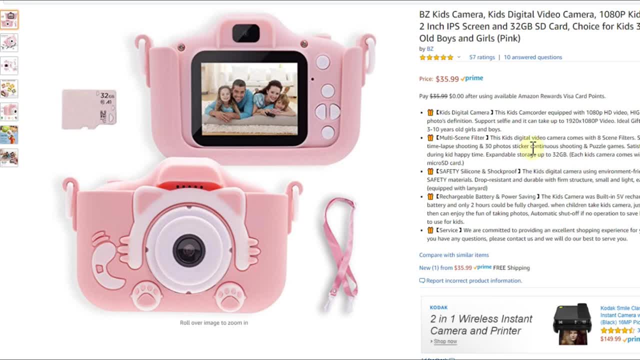 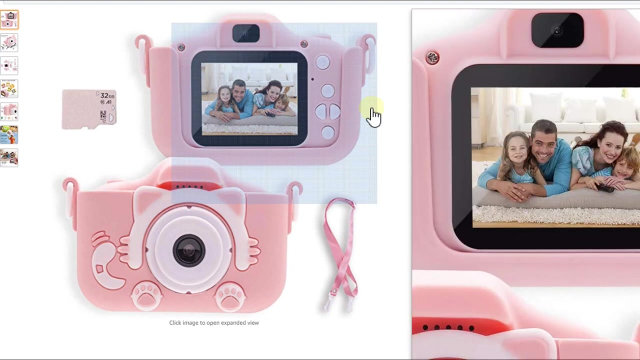 mean you get a lot for the 35, but please don't get deceived about this review: 93 five-star reviews and just uh, yeah, very few four-star reviews and nothing below that. and yeah, this is completely dishonest. i mean, this camera is i mean- i'm not saying it's junk, i mean 32 dollars. yeah, i mean you get the card. you. 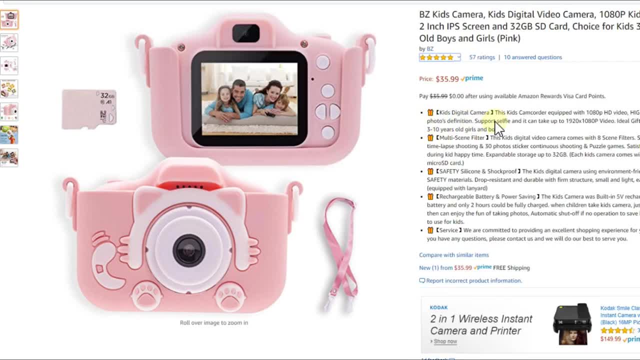 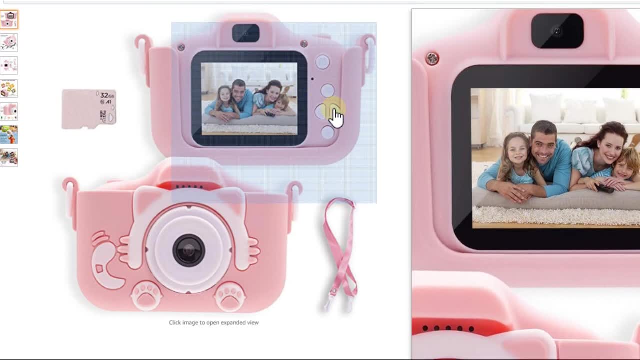 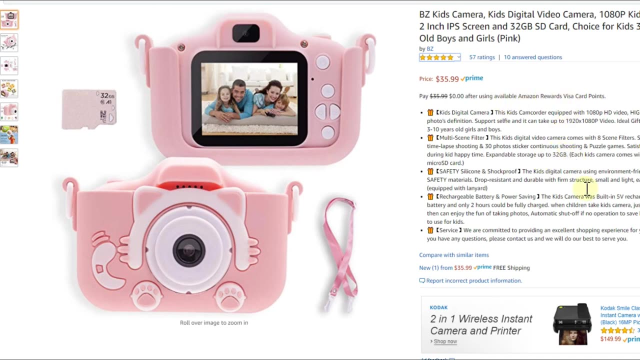 can get something which kids can play around. they can make basic pictures and videos. they get even built in gaming. they learn something. yeah, i mean, but still i'm not saying you cannot buy this for a three-year-old maybe. but at least i think you have to really promise, if you buy something like this, to